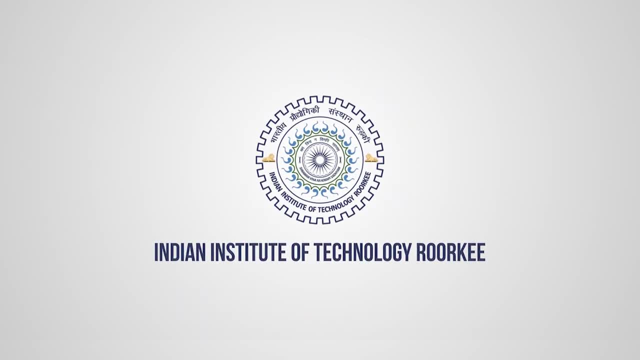 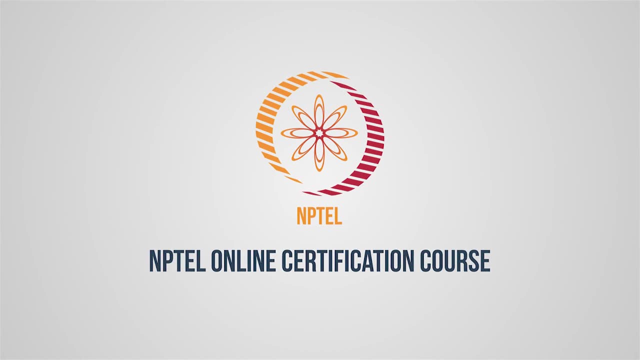 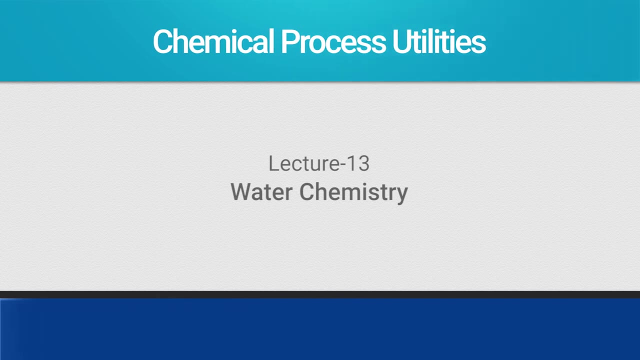 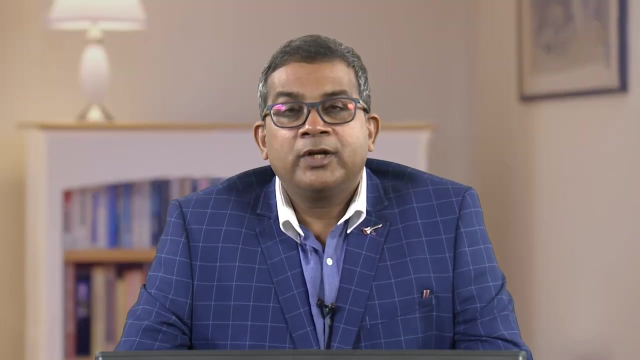 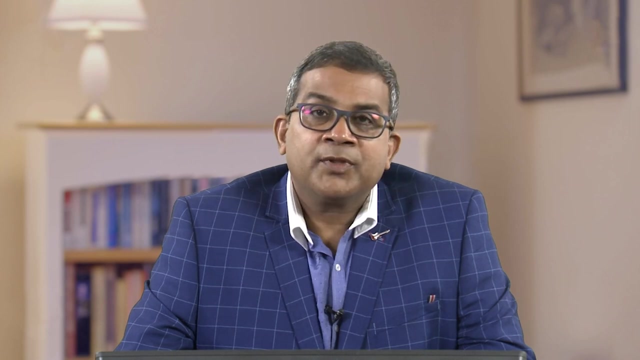 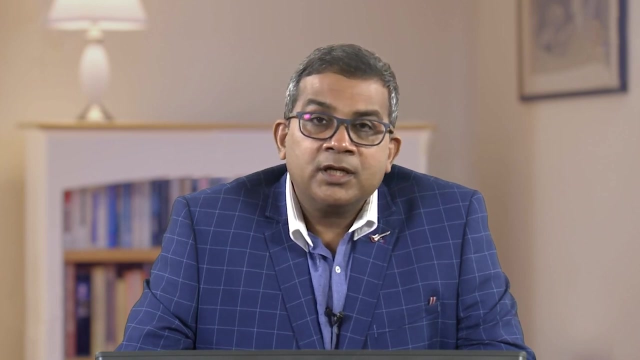 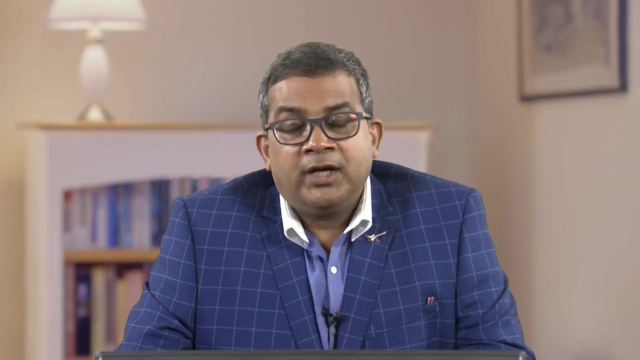 Welcome to the next chapter of Water Chemistry Under the Ages of Chemical Process Utilities. Now we have covered about. we were discussing about the source of water. we were discussing about the various water chemistry in which we have discussed the various contaminants present in the water. Now we had already discussed that, how these contaminants are. 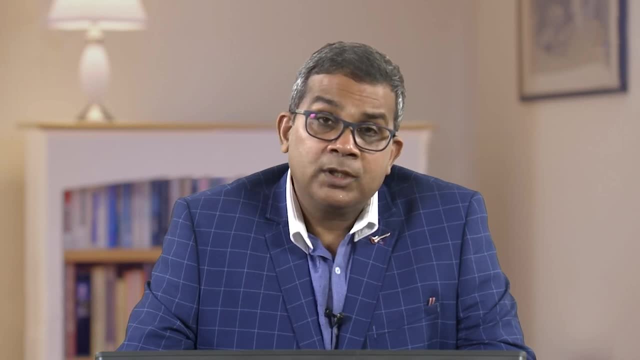 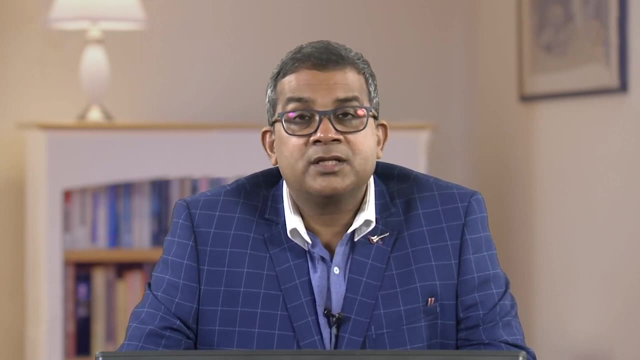 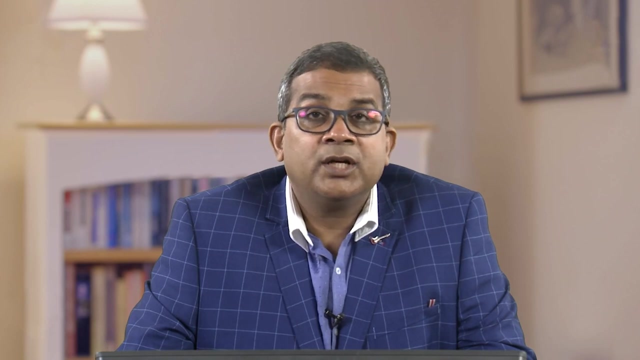 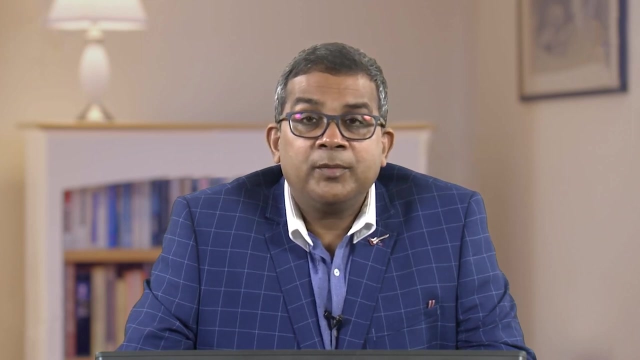 important, especially the determination and removal, because it may seriously affect the process. It may seriously affect the presence of these contaminants, may seriously affect the energy efficiency economical aspect and sometimes it may cause the wear and tear to the equipment and, moreover, they may catalyze the reaction so that any unwanted product may become the 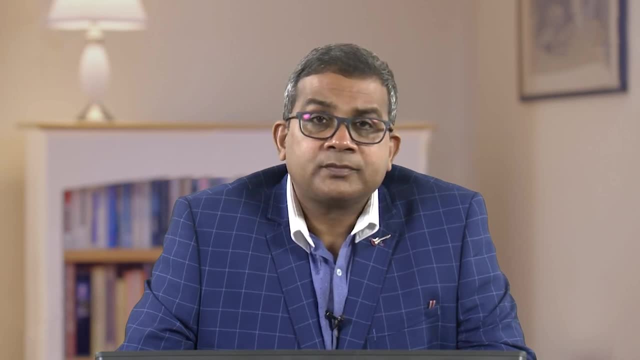 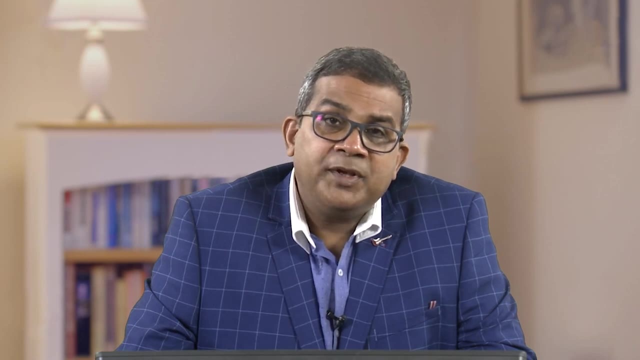 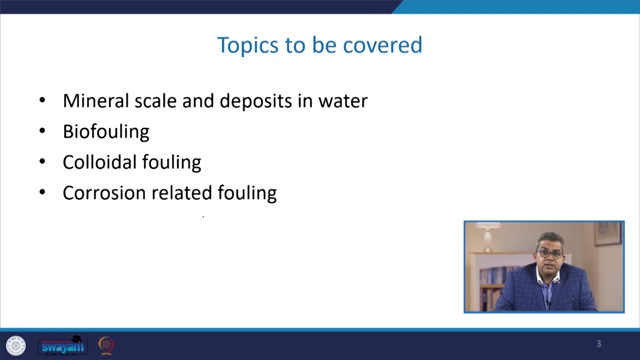 part and parcel of our chemical processes. Now, in this particular lecture, we are going to cover about the concept of mineral scale and deposits. Now we will have an idea about the biofouling. we will discuss about the colloidal fouling. 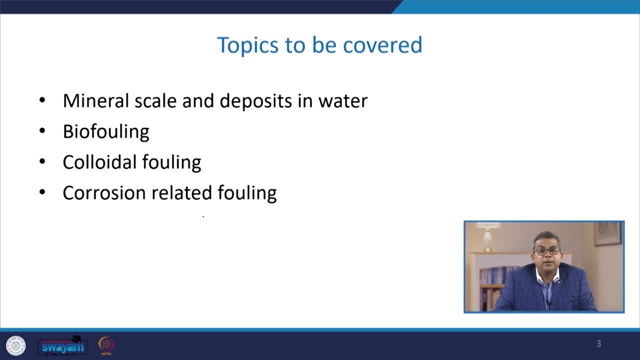 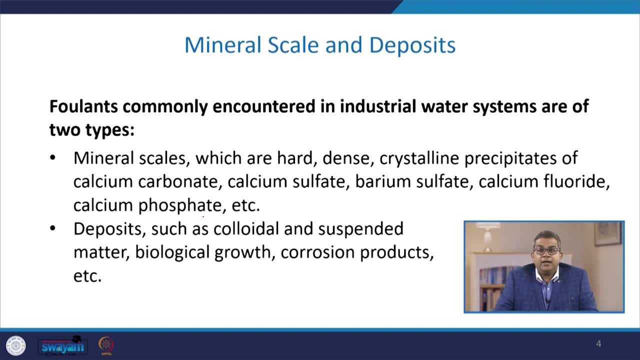 we will have a discussion about the corrosion related fouling. Now let us have the first thing in picture, that is, the mineral scale and deposits. Now foulants commonly encountered in industrial water system are of two types. basically, there are two types. 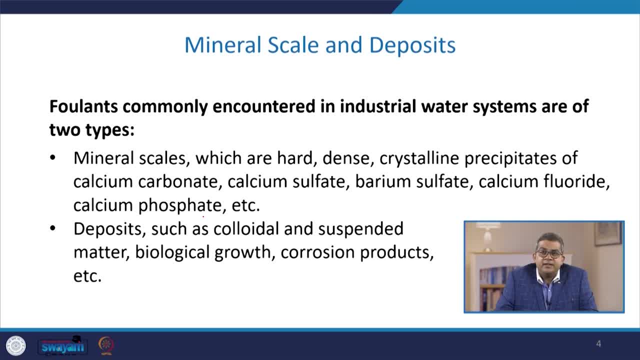 One, the mineral scale. The mineral scales which are hard, dense, crystalline precipitates of calcium carbonate, calcium sulphate, barium sulphate, calcium fluoride, calcium phosphates, etc. So we are discussing so many chemicals etc. but they are very much important. 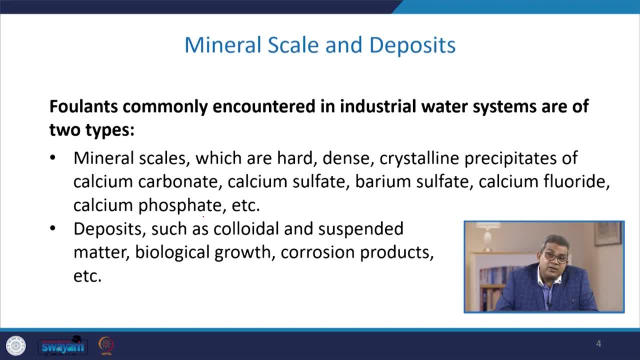 The knowledge, the concentration there, sometimes the controlled removal. all these things are essential Now, second is the deposits, like colloidal fouling, Colloidal fouling Like colloidal or suspended matters, biological growth, corrosion products, etc. 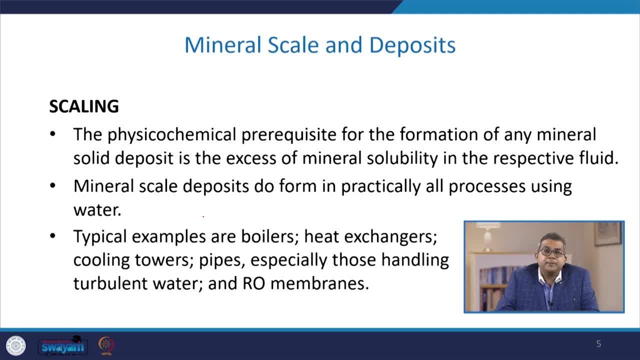 So first we will discuss about the scaling. This is the physicochemical prerequisite for the formation of any mineral solid deposits in the excess of mineral solubility in respective fluid. Now mineral scale deposits do form in practically all processes. They may be of different sizes. 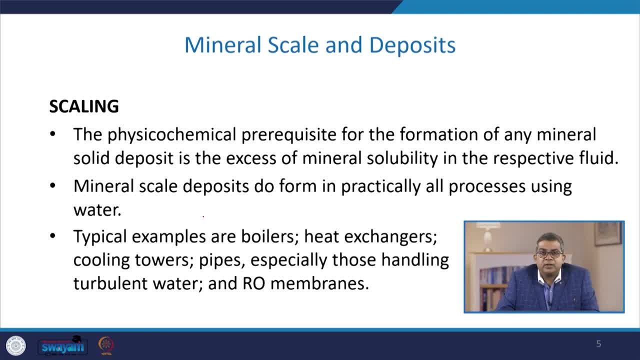 They may be of different sizes in the process. So the mineral scale deposits do form in practically all processes, processes using water. We can enlist several examples: boiler, heat exchangers, cooling towers, pipes- especially those handling turbulent water- or reverse osmosis membranes, etc. 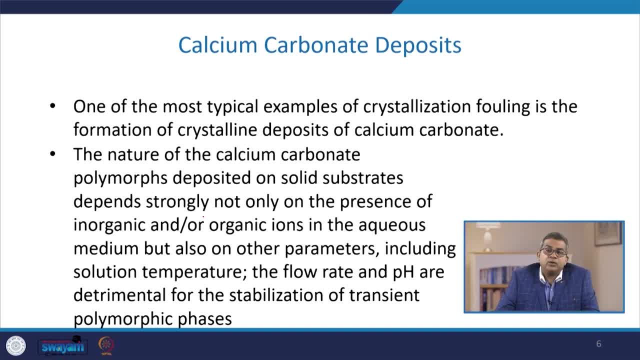 One thing is that scales. they do not offer any kind of a heat effect, but they hinder the smooth passage of the heat transfer, so that is very important. Now let us have a discussion about the calcium carbonate deposits, one of the most typical. 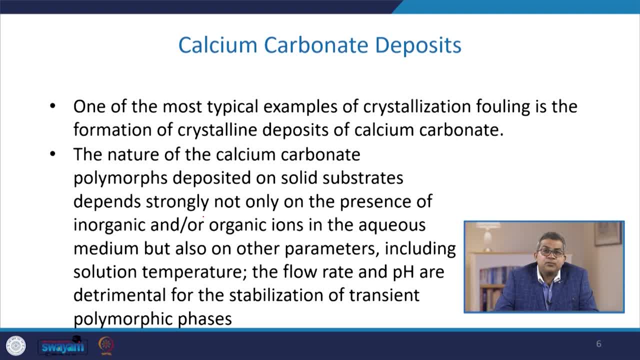 example of crystallization falling is the formation of crystalline deposits of calcium carbonate. Now, the nature of calcium carbonate polymorphs deposits on the solid substrate depends strongly not only on the presence of the inorganic, or you can say the organic ions, The organic ions in the aqueous medium, but also on other parameters like the solution. 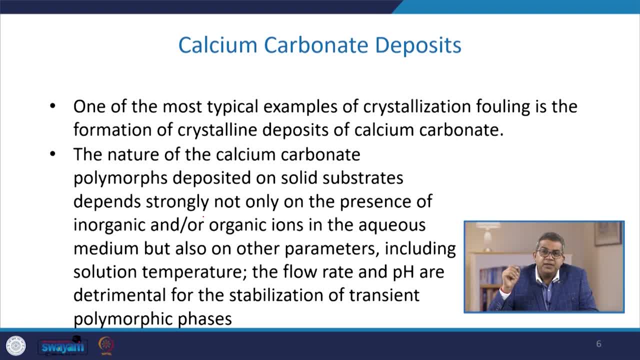 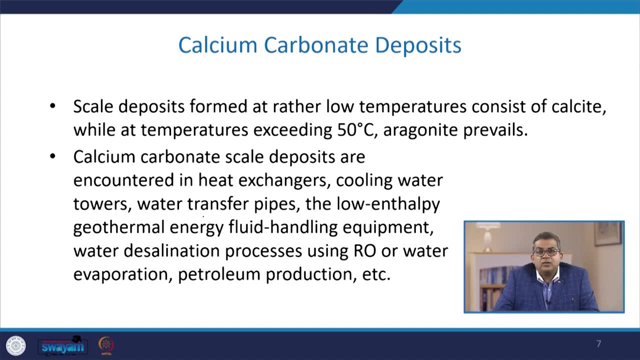 temperature, the flow rate, the pH. These are the detrimental for the stabilization of transient polymorphic phases. Scale deposits, usually formed at rather low temperatures, consist of calcite, While the transition of calcium carbonate deposits is considered to be the most important of the 3 types. 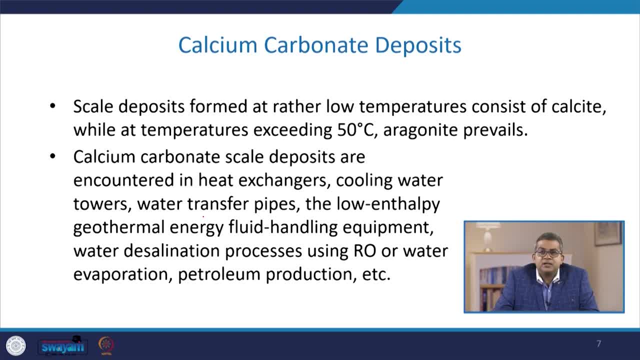 temperature exceeding at 50 degree Celsius, the aragonite prevails. Calcium carbonate scale deposits are encountered in heat exchangers, cooling water towers, water transfer pipes, the low enthalpy geothermal energy, fluid handling equipments, water desalination. 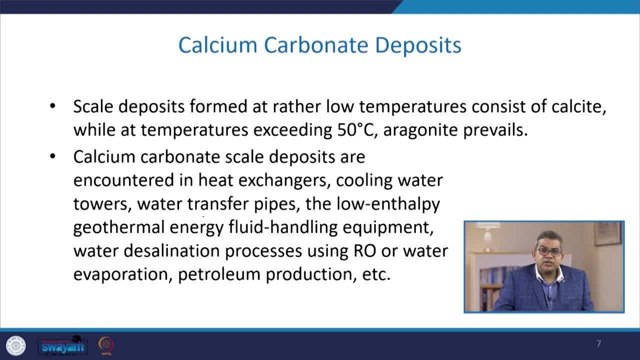 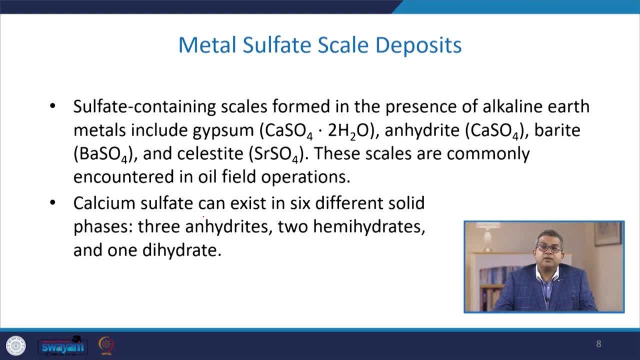 processes using RO or water evaporation, petroleum production, etc. Now let us discuss about the metal: sulfate scale deposits, Sulfate containing scales formed in the presence of alkaline earth metal. this includes the gypsum, a basic formula: CaSO4- 2H2O anhydride. that is CaSO4. 2H2O anhydride- that is CaSO4. 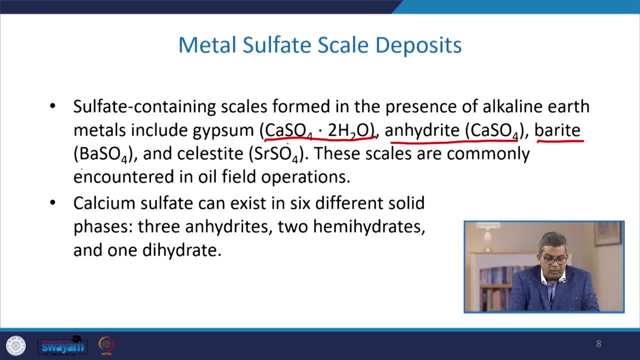 2H2O, barite, or sometimes referred as barium sulfate, BaSO4, celestite, that is, SrSO4.. So these scales are commonly encountered in oil field operations. So we need to find out, we need to know the concentration and then we need to treat accordingly. 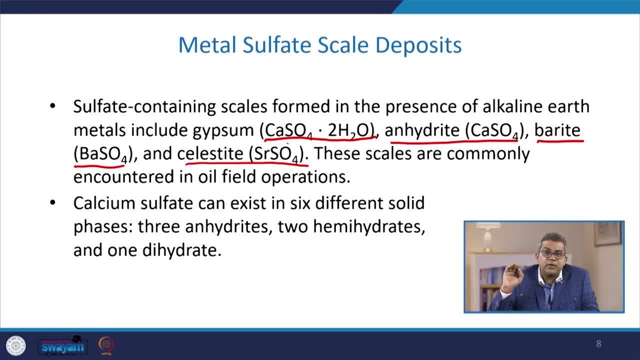 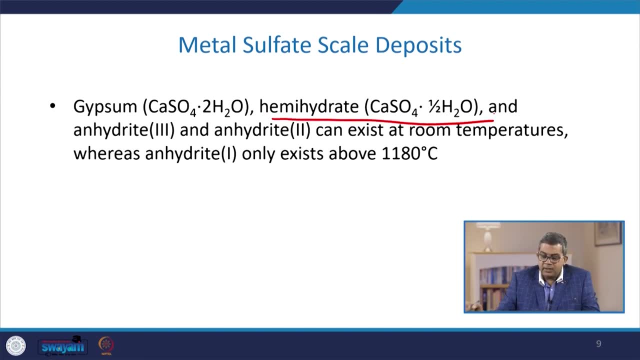 Now calcium sulfate can exist in 6 different solid phases: 3 anhydrides, 2 hemihydrides and 1 dihydrides. Gypsum or hemihydrides having the chemical formula of CaSO4, 1H2O and anhydride 3 and 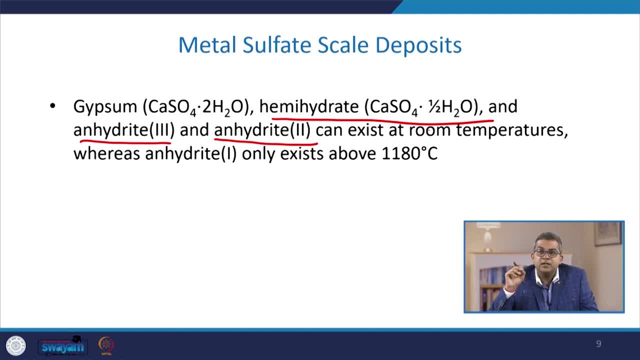 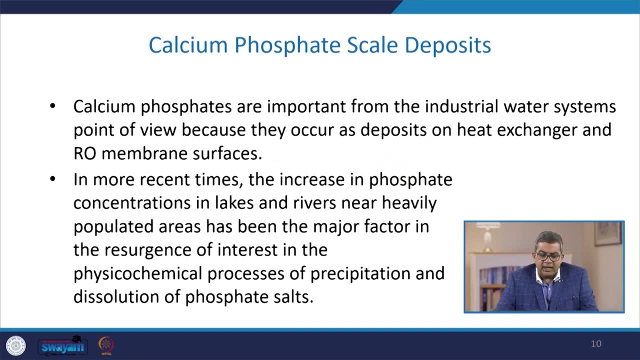 anhydride 2, they can exist at room temperature, where anhydride 1 only exists above the temperature of 1180 degree Celsius. So this is the concentration. Now let us have a discussion about the calcium phosphate scale deposition. 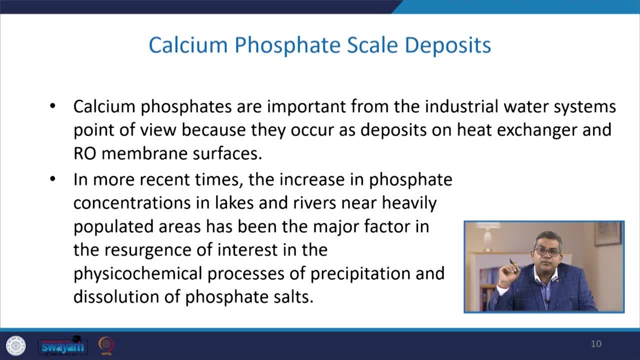 Now calcium phosphates. they are important from the industrial water system point of view if we talk about because they occur as deposits on heat exchanger and reverse osmosis membrane surface. So they clog the pores of these reverse osmosis membrane. 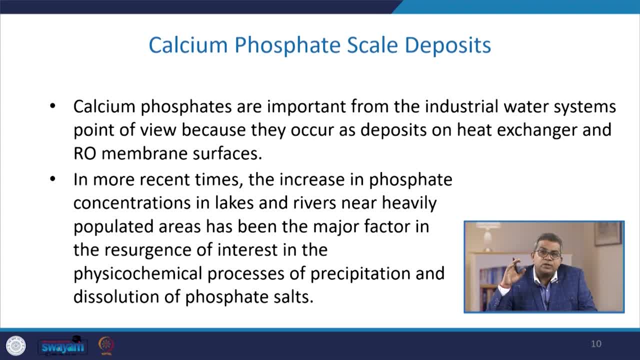 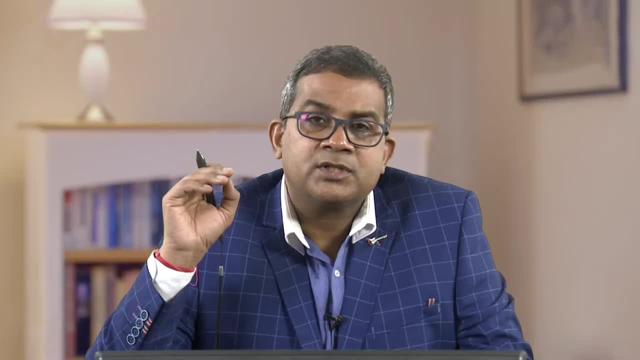 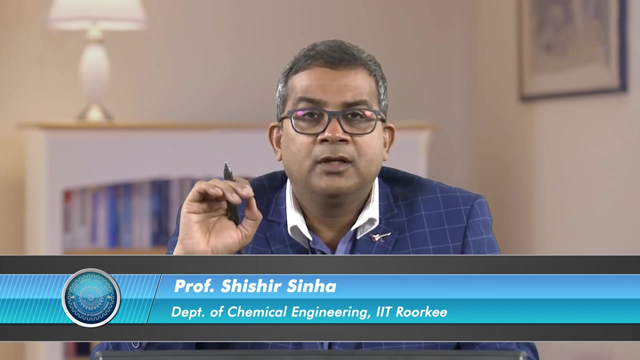 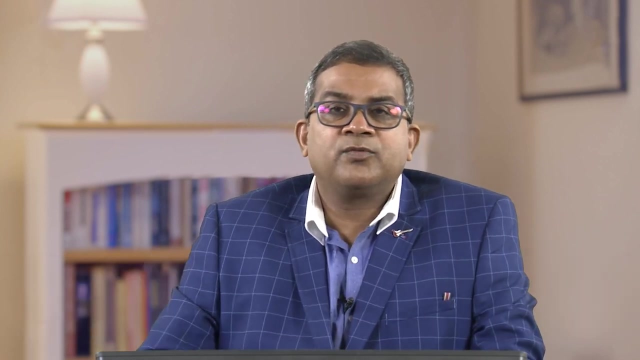 In more recent times, the increase in phosphate concentration in lakes and river near heavily populated area. this has been the major factor in resurgence of interest in physicochemical processes of precipitation and dissolution of phosphate salt. Well, despite of continuous transport of phosphate iron into lake, the phosphate concentration 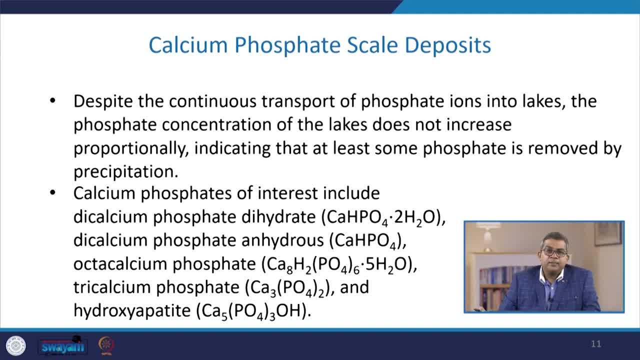 of the lake does not increase proportionally now, indicating that at least some phosphate is removed by precipitation. calcium phosphates of interest include dicalcium phosphate dihydrate having the chemical formula of CaHPO4- 2H2O. Why are they únicado to a Christmas? 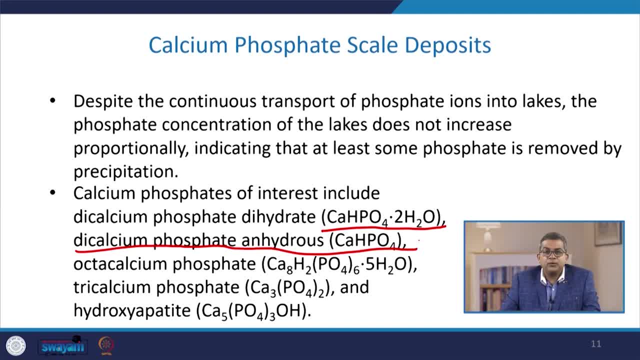 anhydrous, that is, CaHPO4, octa. calcium phosphate, C8H2PO4 whole 6, 5H2O. tricalcium phosphate, Ca3PO4 whole twice and hydroxytide Ca5PO4 whole thrice OH. 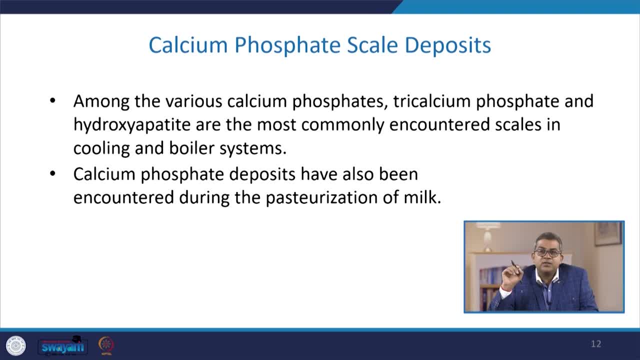 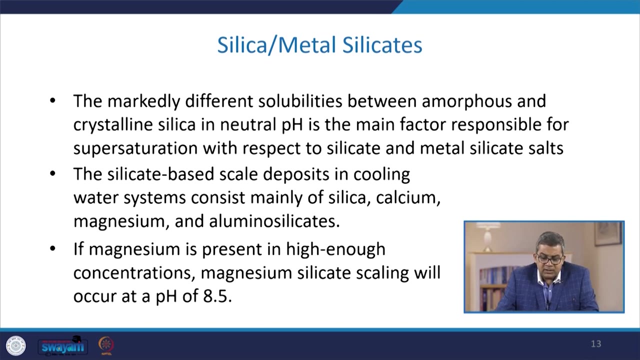 Now, among the various calcium phosphate, tricalcium phosphate and hydroxytide, they are the most commonly encountered scales in cooling and boiling system Calcium phosphate deposits. they have also been encountered during the pasteurization of mill. Now let us have a discussion about the silica metal- silicates. 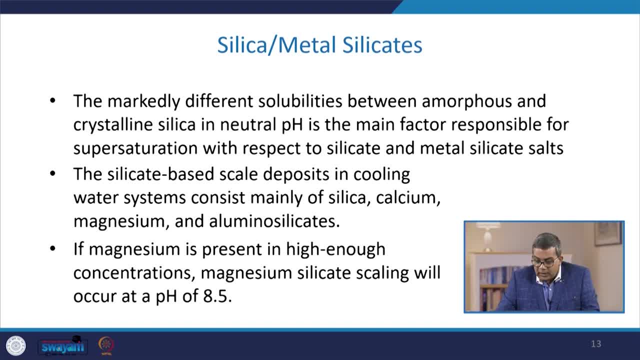 The significant different solubilities between amorphous and crystalline. silica in neutral pH is the main factor which is responsible for super saturation with respect to silicate and metal silicate salts, The silicate based scale deposits in cooling water system. it consists mainly of silica. 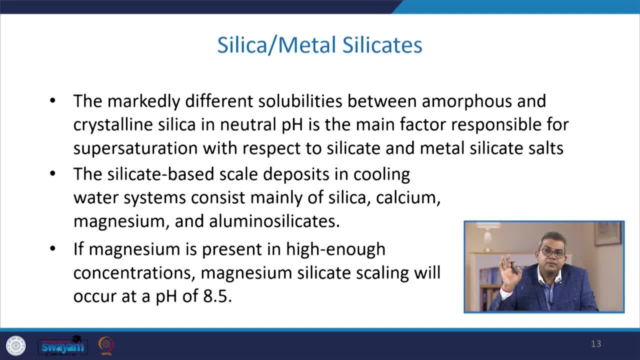 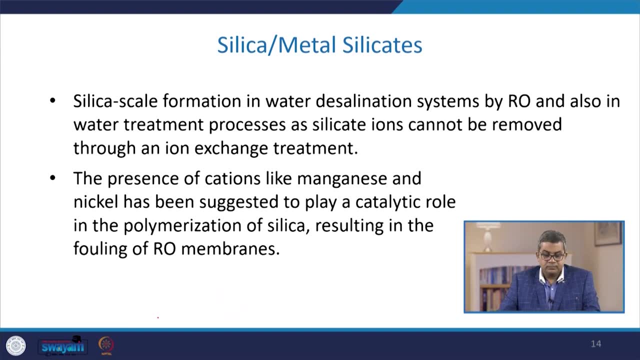 calcium, magnesium and alumino silicate. Ah, If you see that magnesium is present in high enough concentration, magnesium silicate scaling will occur at a pH of 8.5.. Silica scale formation in water desalination system by reverse osmosis and also water treatment. 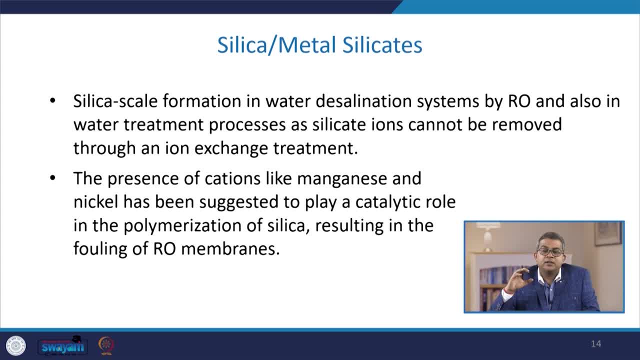 processes as silicate ion. It cannot be removed through an ion exchange treatment. So it cannot be removed through ion exchange treatment. The presence of cations like manganese and nickel. this has been suggested to play a catalytic role in the polymerization of silica. 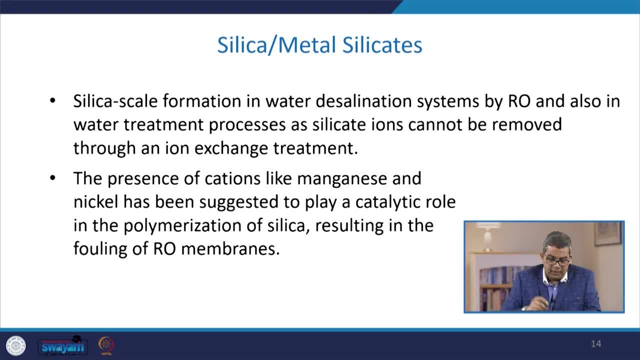 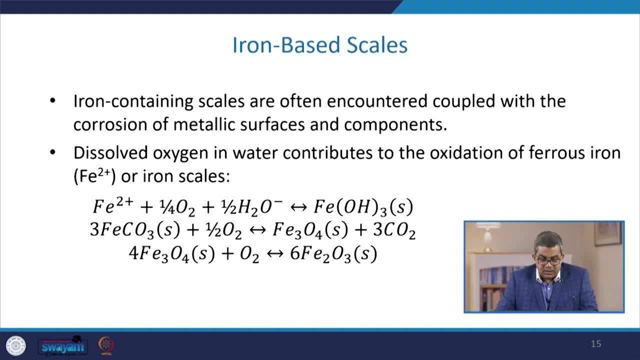 This may result in the falling of reverse osmosis membrane. Now let us have a discussion about the iron based scales. Now iron containing scales. they are often encountered coupled with corrosion on the surface. Now let us have a discussion about the series of iron based scales. 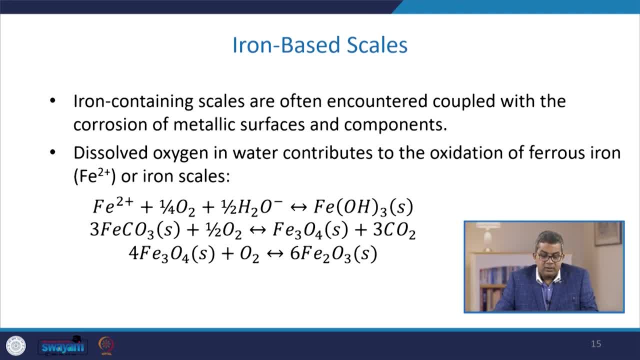 of metallic surfaces and components, Dissolved oxygen in water. sometimes it contributes to the oxidation of ferrous ion, Fe2 plus or iron scales. Now these are the some of the chemical reactions, like Fe2 plus plus quarter oxygen plus half 4 H2O ion, FeOH3, whole thrice, then FeCO3 in the solid phase, half O2 gives the Fe3O4 plus. 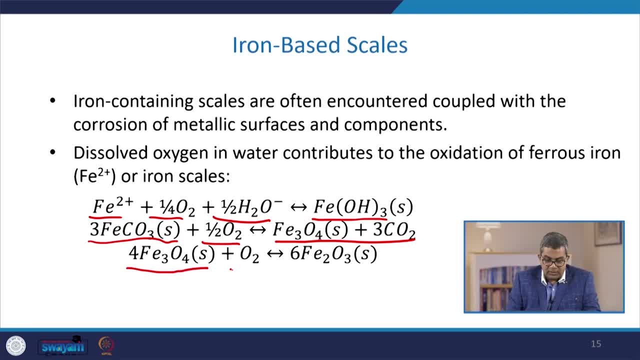 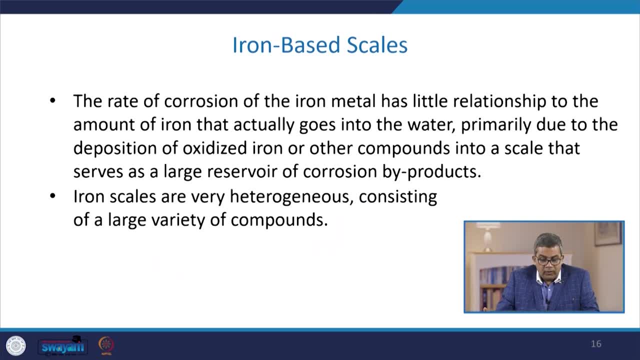 3 CO2 or Fe3O4 plus O2. this gives the 6 Fe2O3.. Now when we talk about the further, about the iron based scales, the rate of corrosion of the iron metal, It has the literal relationship to the amount of iron that actually goes into the water. 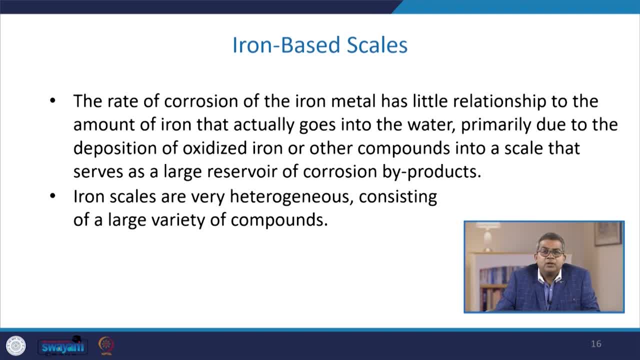 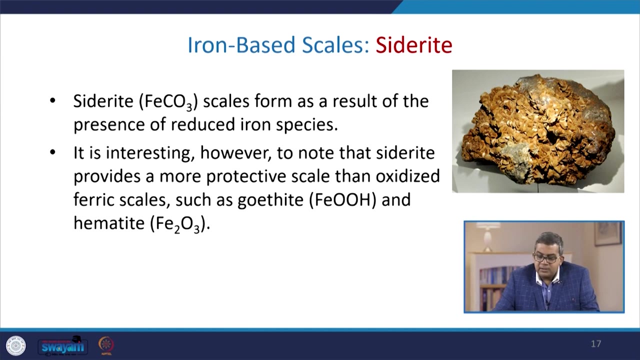 primarily due to the deposition of oxidized iron or other compounds into a scale that serves a large reservoir of corrosion byproduct. Now iron scales are very heterogeneous, consisting of a large variety of compounds. Now, one of the iron based scale that is siderite. now this siderite is FeCO3 scale we can have 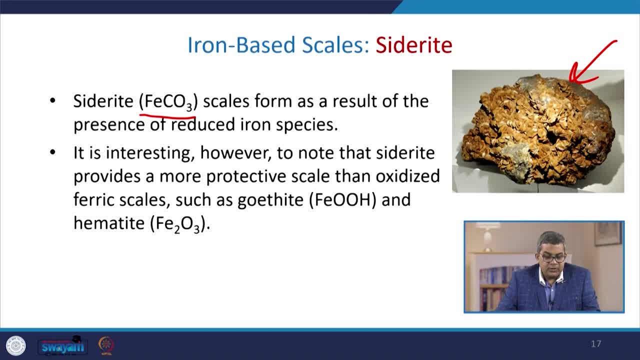 a look. this is this picture where the scales form as a result of presence of reduced iron species. Now it is interesting, however, that to note that siderite provides a more protective scale than oxidized ferric scales such as FeCO3.. Now we can have a look. this is this picture where these scales form as a result of presence. 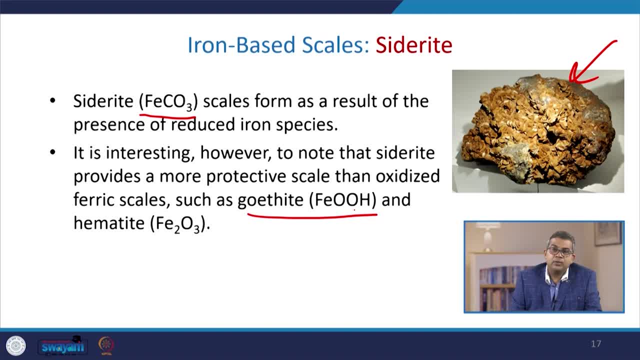 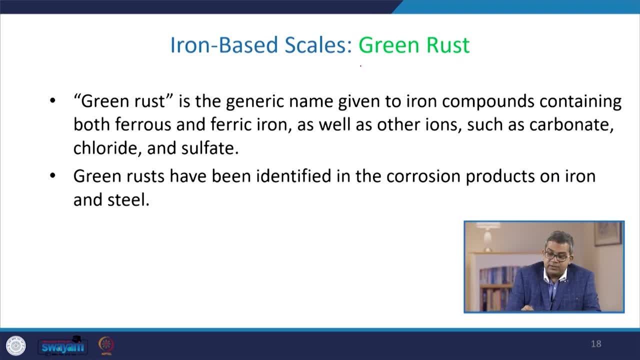 of reduced iron species. So here there is a graph here. So green rust, that is a graph here, where this is the geotite, that is, FeOOH and hematite Fe2O3.. Now green rust is the generic name given to the iron compound containing both ferrous 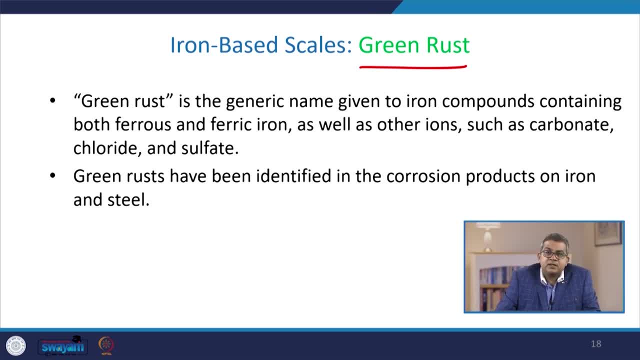 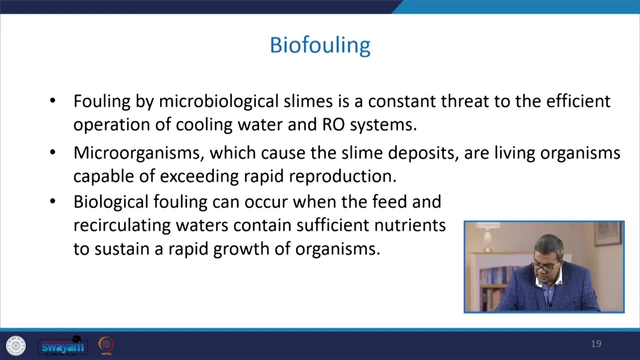 and ferric ion, as well as ions such as carbonate, chloride and sulfate. Now this green rust have been identified in the case of silicon- that is the generic name, the corrosion product on iron and steel. Now let us have a discussion about the biofouling. 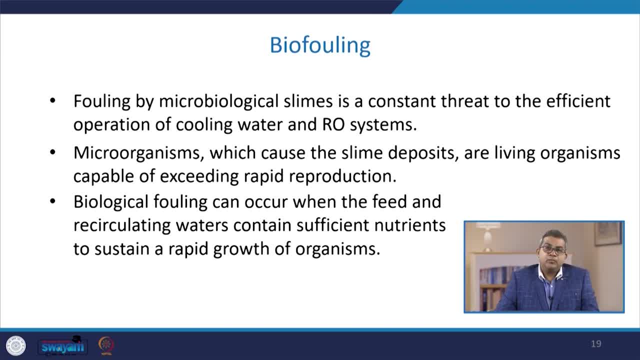 Now this occurs, or fouling occurs by microbiological slimes, is a constant threat to the efficient operation of cooling water and reverse osmosis system Organisms which cause the slime deposit. they are the living organism capable of exceeding rapid reproduction. So the biological fouling. this can occur when the feed and recirculating water contains. 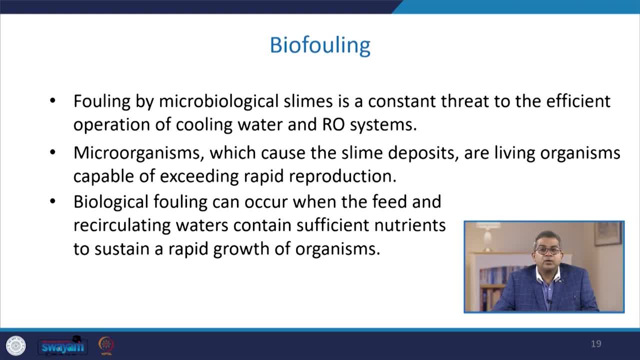 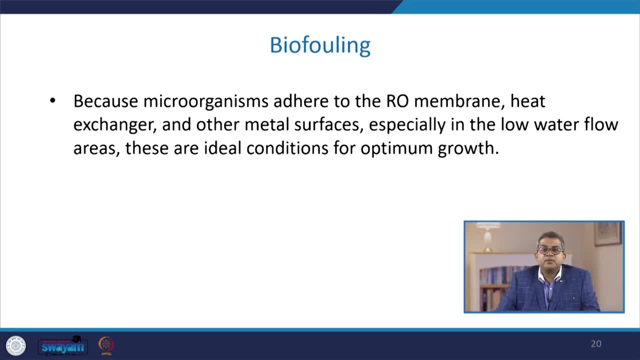 sufficient nutrients to sustain a rapid growth of organism. Now, because of microorganisms adhere to the reverse osmosis membrane, heat exchanger and other microorganisms can cause slimy deposits, Other metal surfaces, especially in the low water flow area. these are ideal condition. 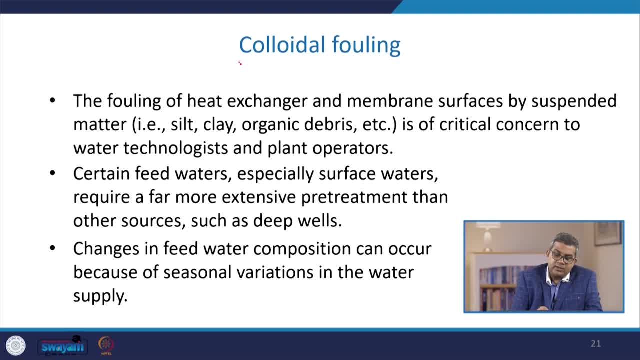 for the optimal growth. Now let us have a discussion about the colloidal fouling: The fouling of heat exchanger and membrane surfaces by suspended matter that is maybe silt, clay, organic debris, etc. this is a critical concern to water technologist. 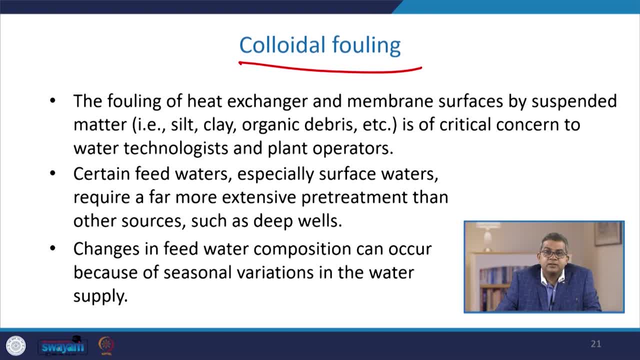 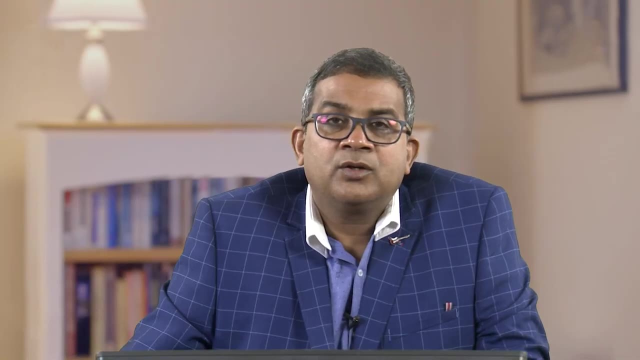 water conditioning persons and plant operators Certain feed waters, especially the surface water. they require a far more extensive pretreatment than other sources such as deep wells etc. Changes in sometimes the feed water composition. it can occur because of the seasonal variation in the water supply. 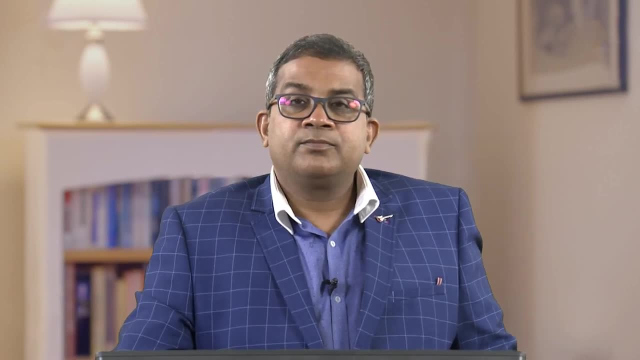 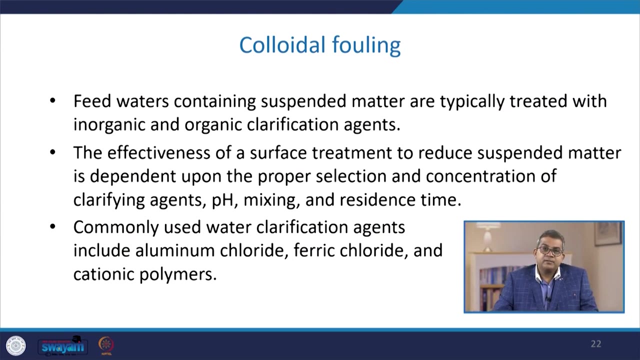 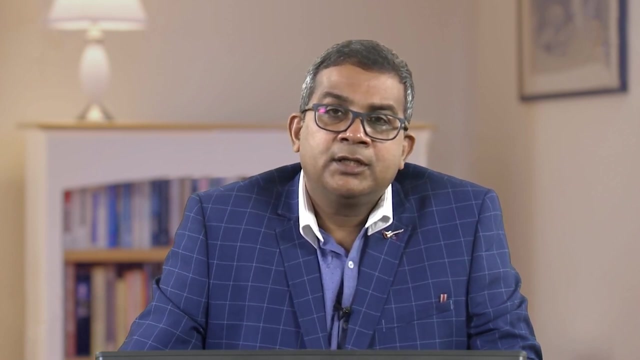 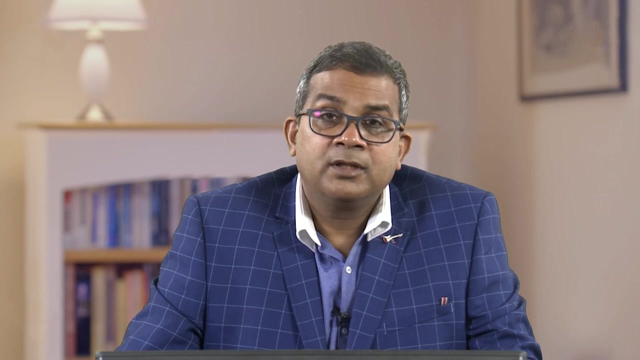 Feed water containing suspended matter. They are typically treated with inorganic or inorganic clarification agents. The effectiveness of surface treatment to reduce suspended matter is usually dependent upon the proper selection and concentration of clarifying agent pH, whatever pH we are using, the mixing, the mixing time and the residence time. 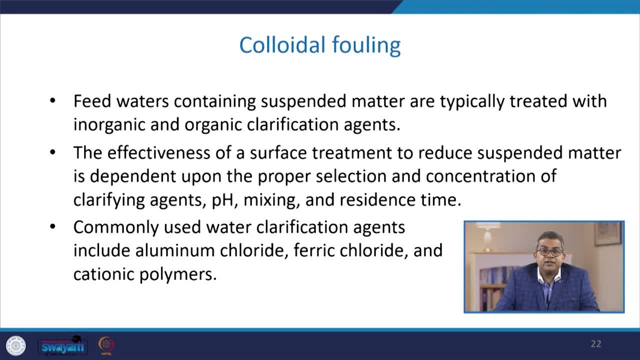 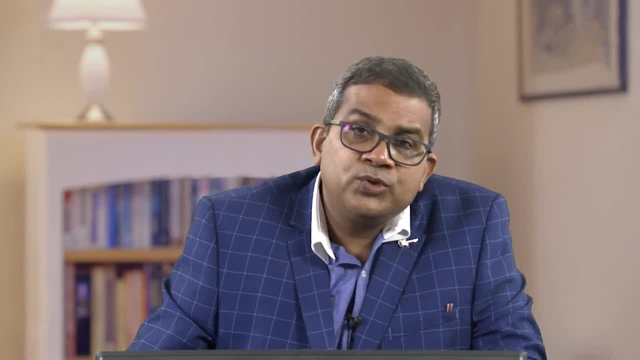 There are a lot of stress in the liquid and the roll-association factor in the liquid, etc. There are certain commonly used water clarification agents, including aluminium chloride, ferric chloride, some of the cationic polymers, etc. They are the commonly used water clarifiers. 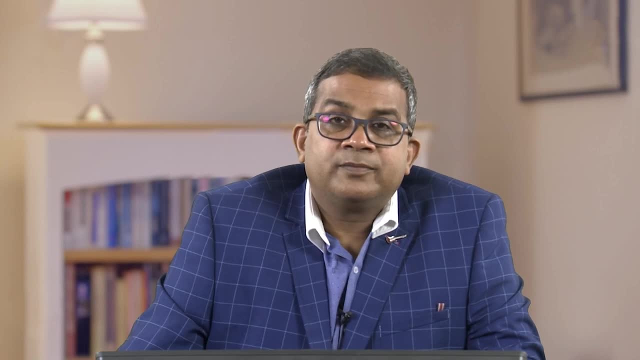 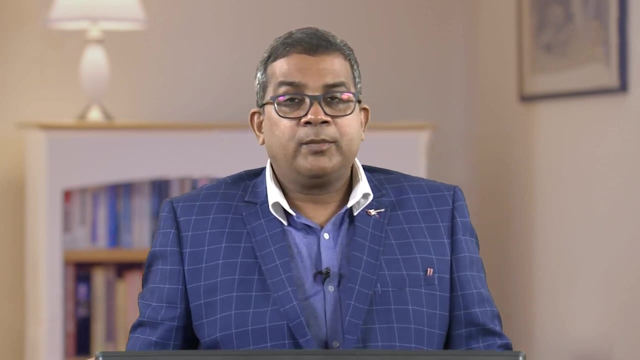 There are certain fouling. they are related to the corrosion. Now, corrosion is a very common phenomena and it usually occurs in all chemical process industries. 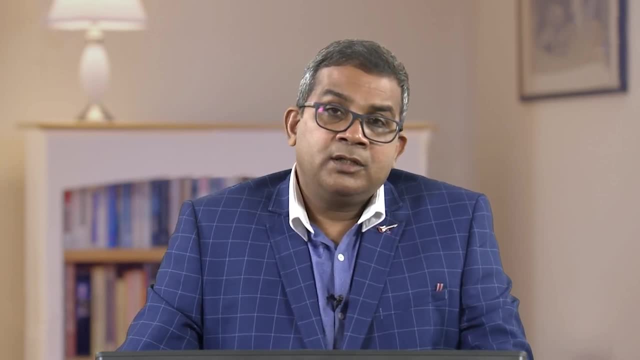 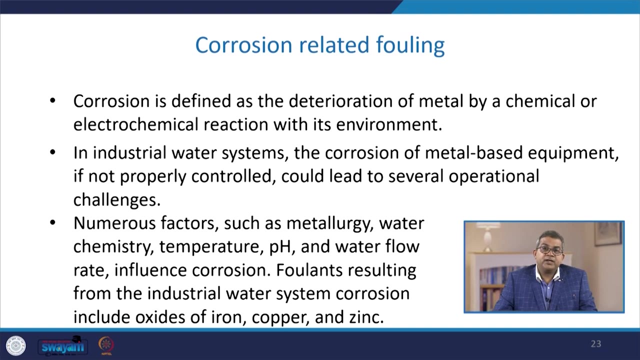 So let us have a brief discussion about the typicalouged description about the corrosion. it is defined as the deterioration of metal by chemical or electrochemical reaction with its environment. So you can see it is a broad spectrum or a broad definition. 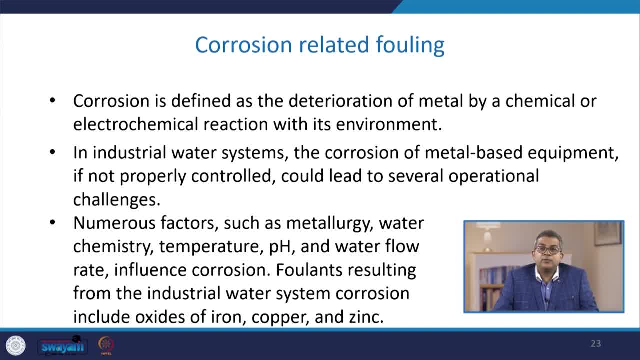 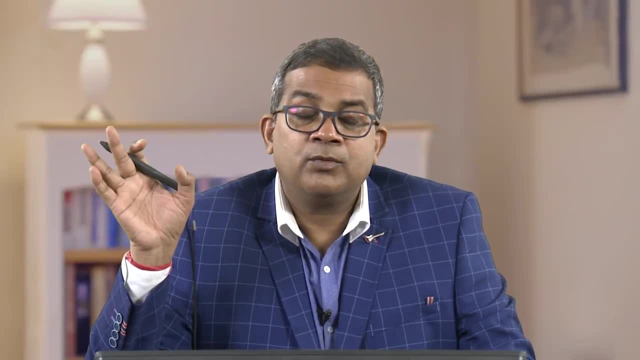 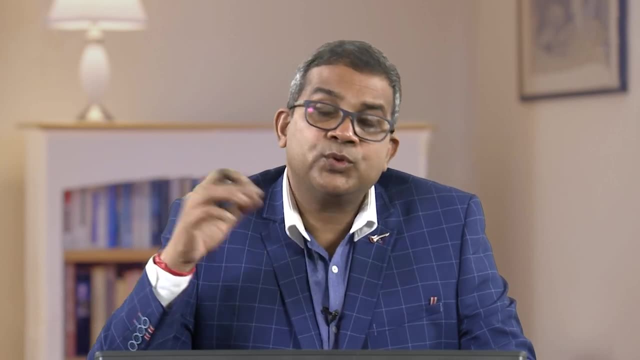 Now, when we talk about the industrial water system, the corrosion of metal based equipment is not properly controlled. if we are unable to control it, this may lead to the several operational challenges and sometimes it may create a serious hazard to the safe environment or safe working condition. apart from the environmental problem, apart from energy issues, 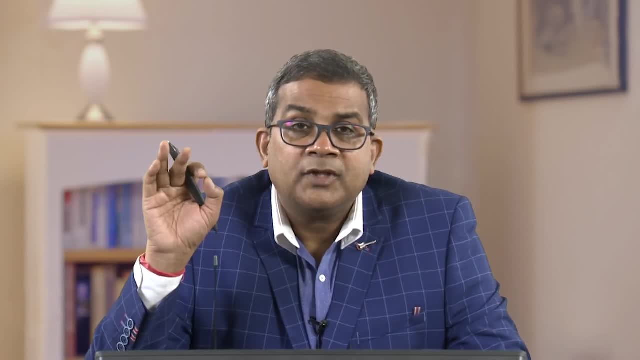 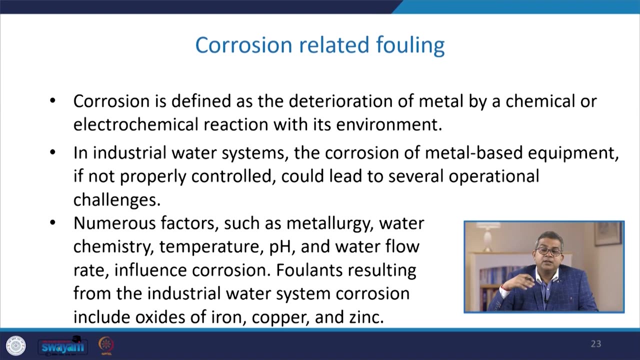 apart from various wear and tears, etc. So numerous factors such as metallurgy, water chemistry, temperature, temperature of the water, knowledge about the pH, water flow rate, they are influencing the corrosion Fall-ends resulting from the industrial water system. corrosion includes the oxide of iron. 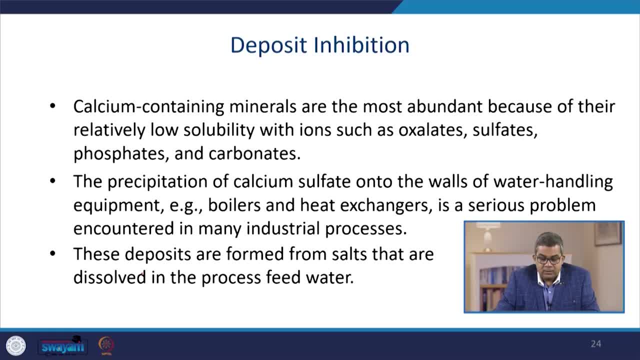 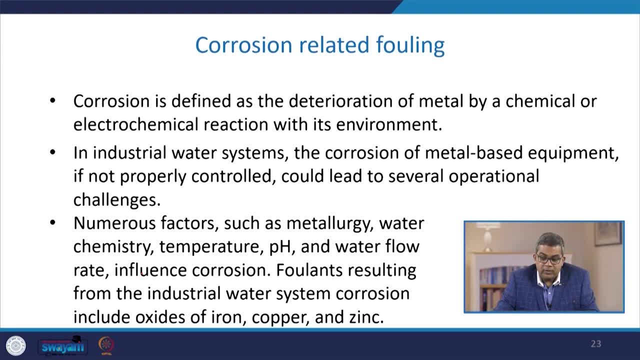 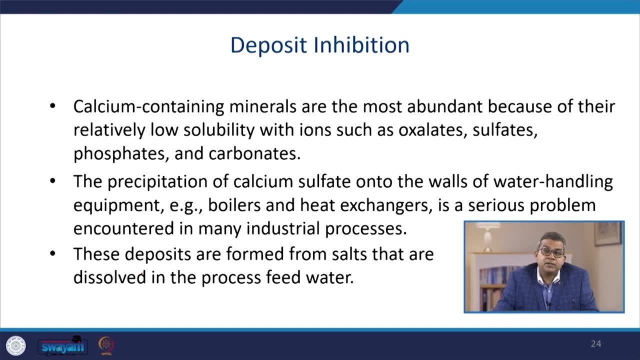 copper zinc. Now let us have a discussion about the deposit inhibition. Now inhibition is again very important because earlier we had discussed about the various kind of falling aspect. Now we understand… Okay, content- that falling is again extremely, you can say- the detrimental for any kind of a. 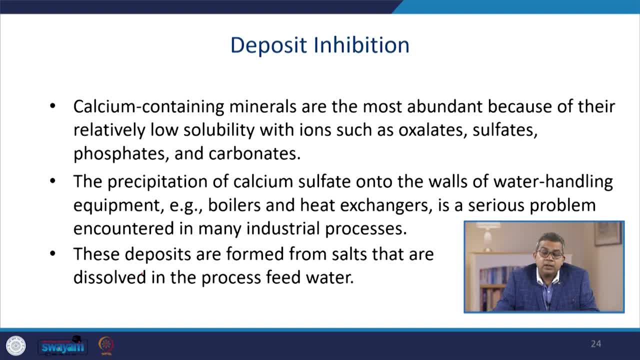 chemical operation. So we need to think about the inhibition of all kind of these deposits, how we can go ahead. what are the surface preparation, what are the different type of chemistry involved in this kind of inhibition, deposit inhibition aspect? So let us have a brief discussion and in due course of time and the subsequent time we 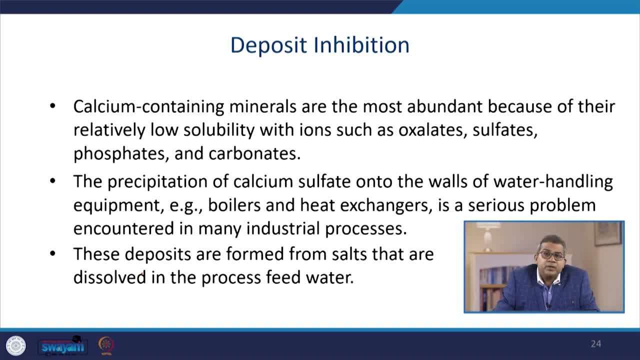 will discuss about this inhibition aspect. Now, calcium containing minerals- they are the most abundant because of their relatively low solubility with ions such as oxalate, sulphates, phosphates, carbonates, etc. Now the precipitation of calcium Calcium sulphate onto the walls of water handling equipments may be. the tube may be. 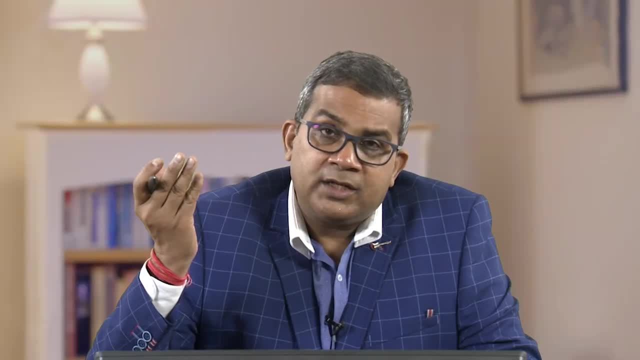 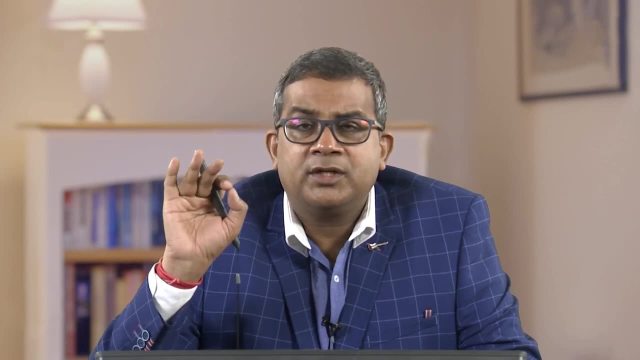 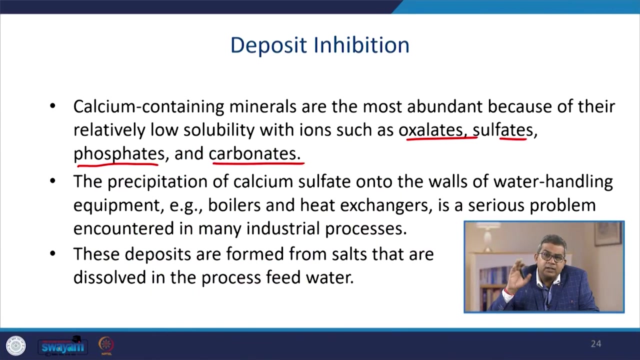 the pipes, etc. these are used in the boiler and heat exchanger. This is a serious problem encountered in various industrial operations. These deposits are formed from salts that are dissolved in the process feed water. I am giving you one example: Like if you repeatedly heat the water. 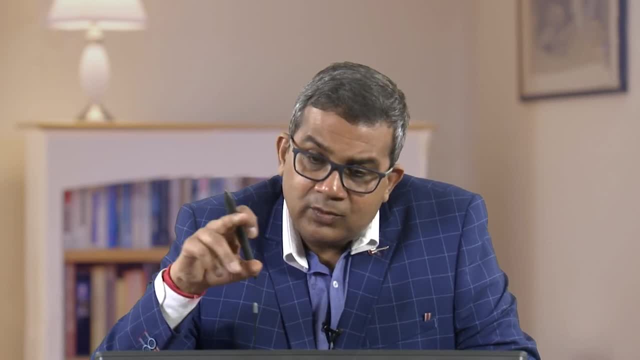 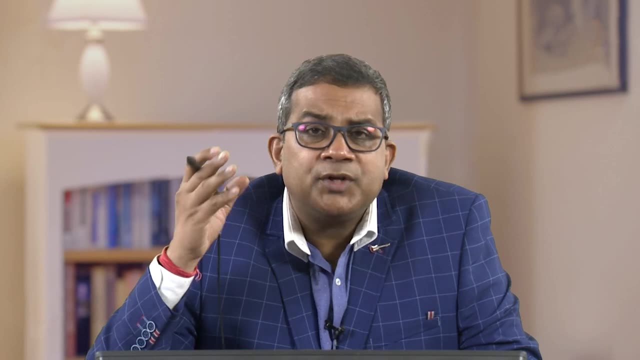 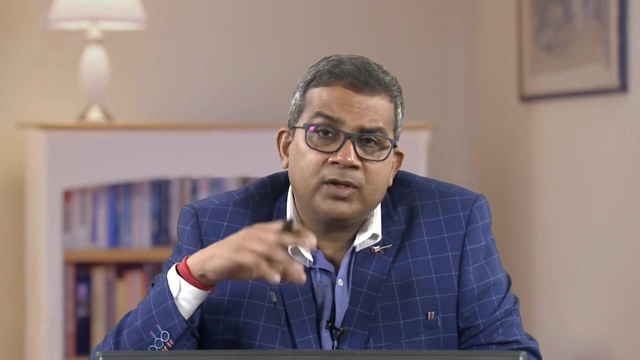 Then the salts may get deposited over the inner lining of other vessel or a pot in which you are depositing. It is a very common phenomena and even you can try in your home also And this sometimes create a very problem because over the period of time, because of the heating, 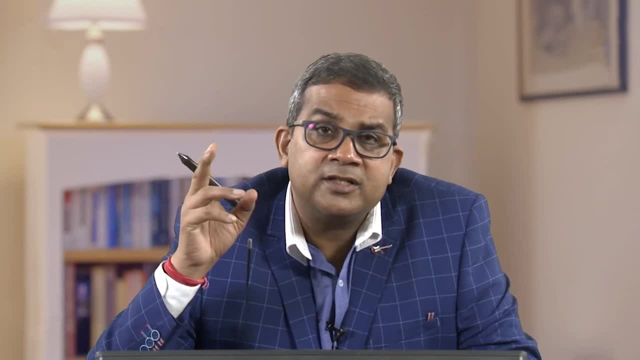 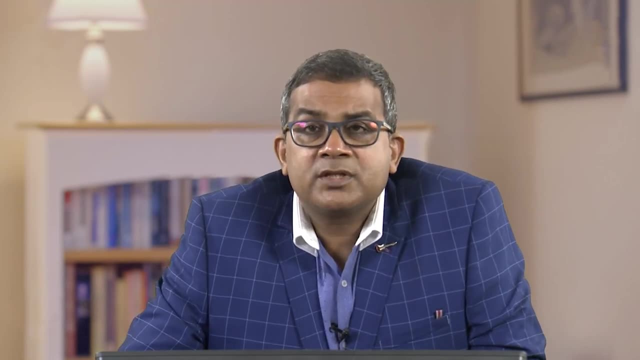 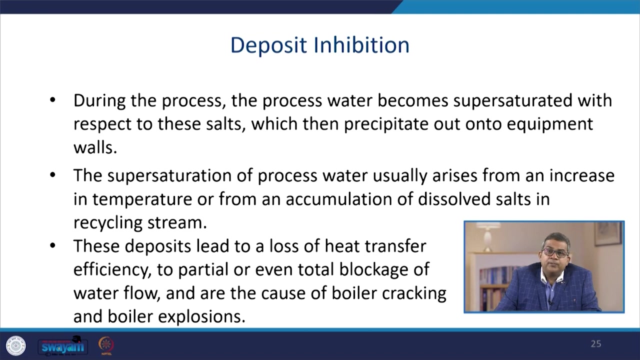 the concentration of these salts keep on increasing, increasing, increasing Now during the process. sometimes the process water, this becomes super saturated With respect to these salts and then they intend to precipitate out into equipment walls, which we I had discussed with the with an example in the previous slide. 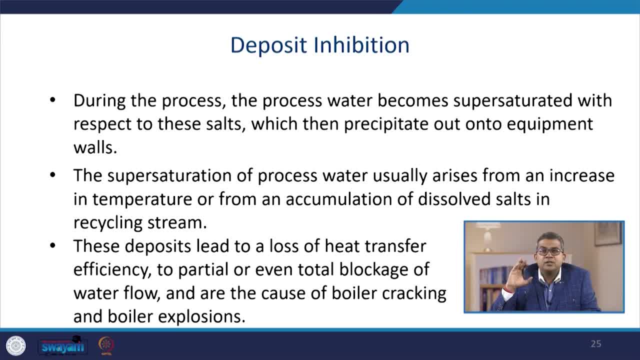 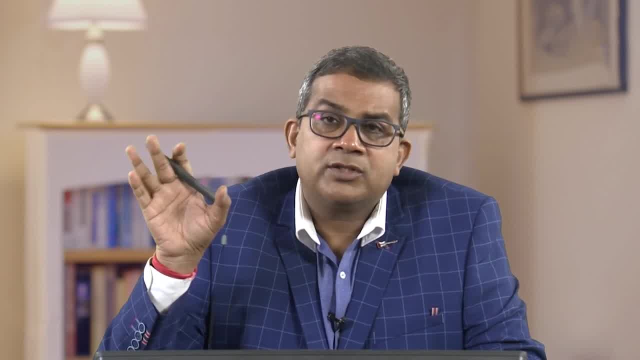 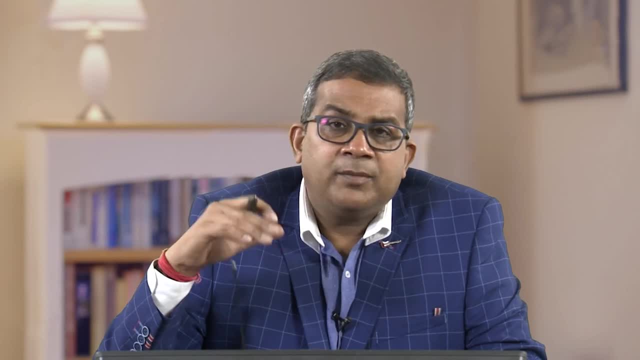 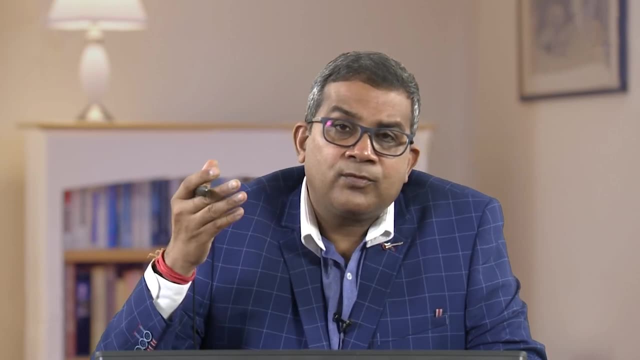 Now the super saturation of process water. This usually arises from an increase in temperature or from an accumulation of dissolved salt in the recycling stream. Now these deposits sometimes lead to the loss of heat transfer efficiency, to partial or even total blockage of water flow, and that cause the boiler cracking, boiler explosion. 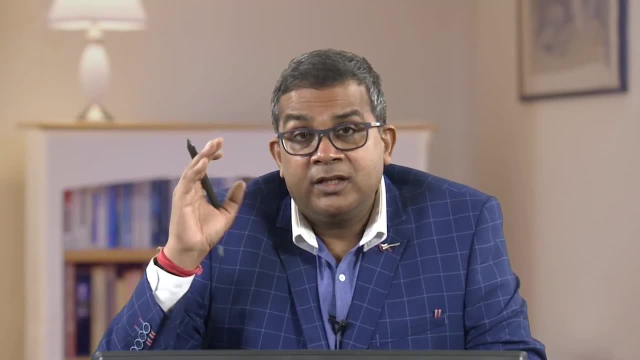 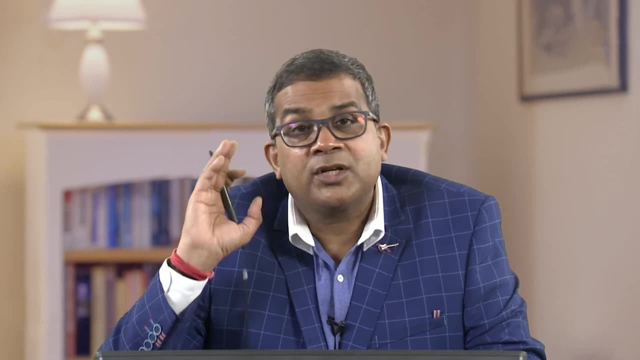 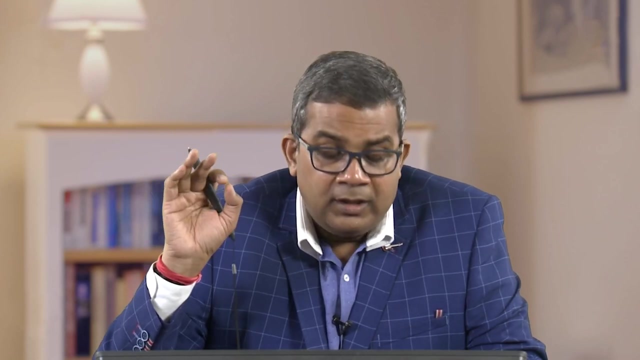 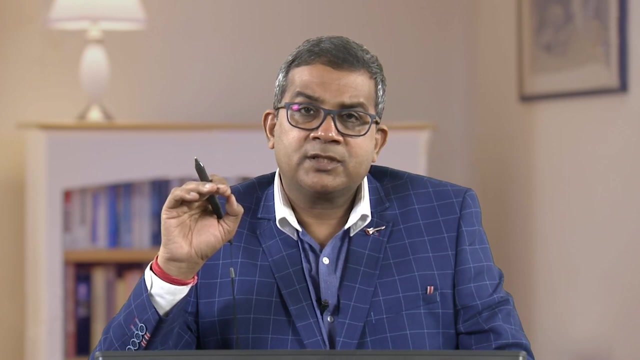 and obviously, when these are things are occurring, then definitely you see that it is a serious hazard, because boiler is not only producing steam but it is a pressure vessel. So it may create a serious problem to the industrial affairs. Thank you. Now scaling, this may be defined as a solid layer. deposition on the surface arises primarily. 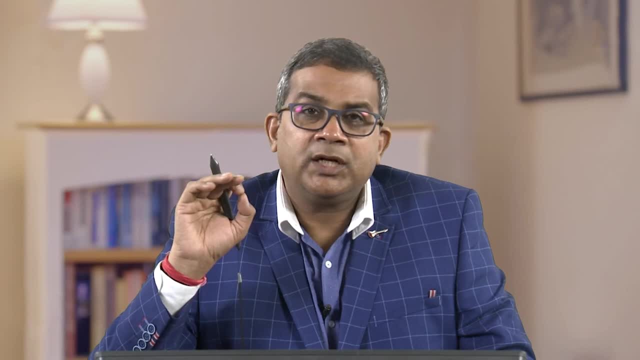 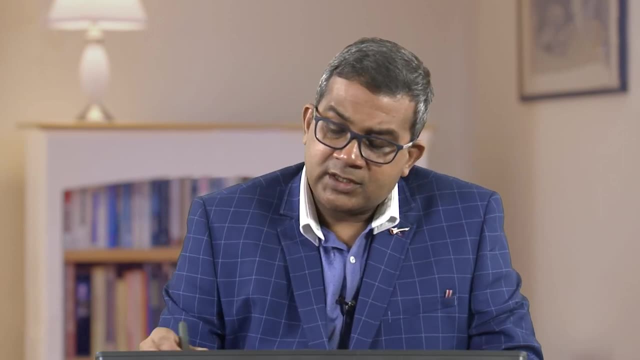 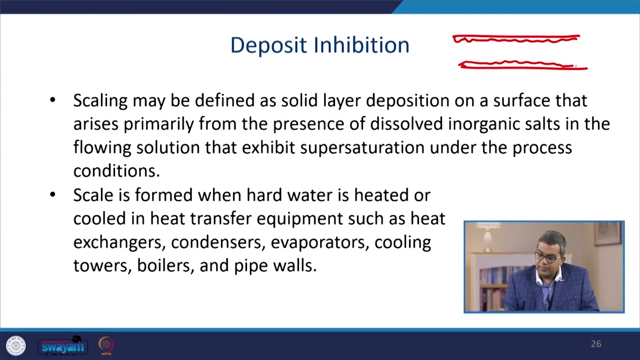 from the presence of dissolved inorganic salt in flowing solution that exhibits the super saturation under the process condition. I am giving you one example. This is the pipeline and scale may get deposited at the inner line. So 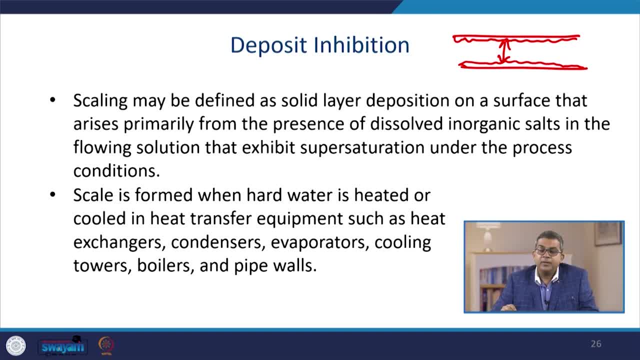 and this prospective inner diameter may reduce. this thereby creates a flow disturbance. This thereby creates the problem in the heat transfer. Similarly, if these tubes are being used in boiler, then again it creates a problem and which we had already discussed in the previous slide. 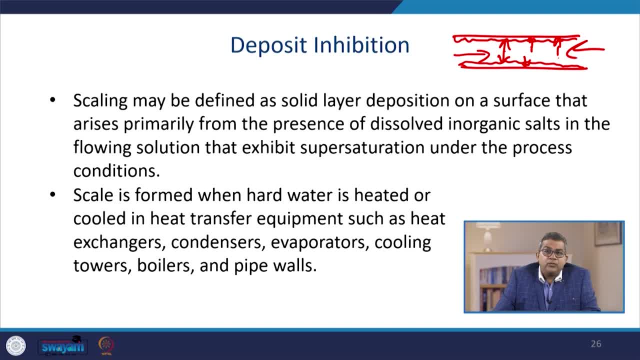 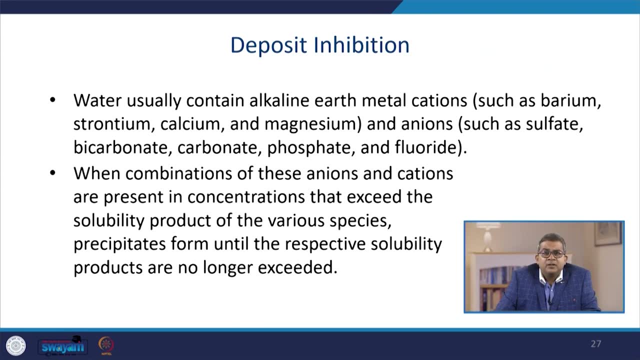 Now scales are formed when hard water is heated or cooled in heat transfer equipment such as heater, heat exchanger, condenser, evaporators, cooling towers, boiler tubes, pipe walls, etc. So water usually contains alkaline earth metal cations such as barium, strontium, calcium. 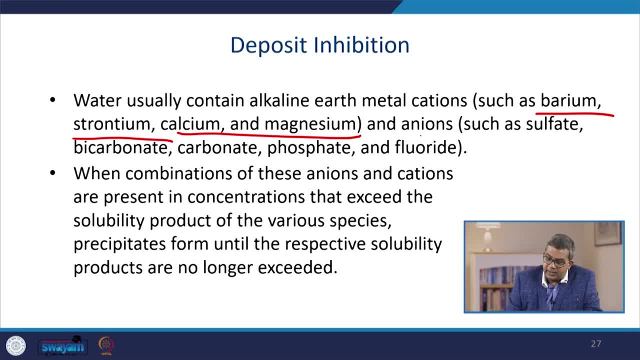 and magnesium, and sometimes anions such as sulphates, bicarbonates, carbonates, phosphate, fluorides. Now, when combination of these anions and cations- they are present in concentration that exceeds the solubility, product of the various species precipitates from form until the respective. 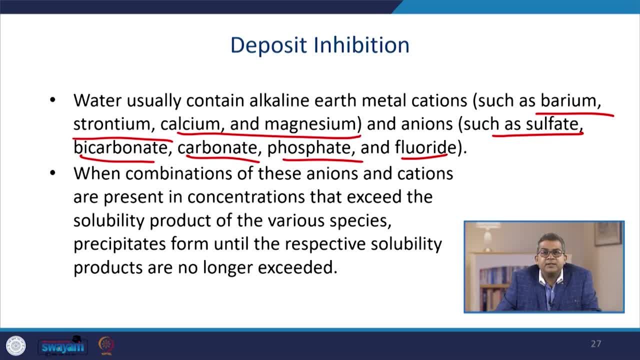 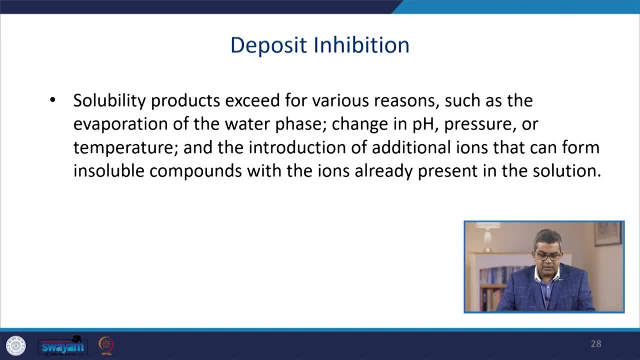 solubility products are no longer exceeded Now. solubility products, this exceeds for various reasons, such as evaporation of water, phase change in pH, pressure, temperature. again you see that the pressure and temperature they are having the wide range and sometimes the introduction of additional ion that can. 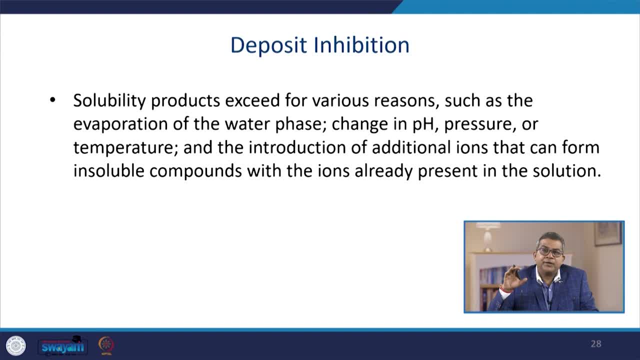 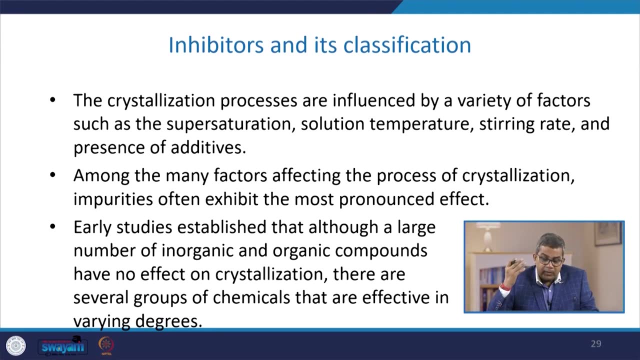 form the insoluble compounds with the ion already present in the solution. So every time, do not think that these are the negative aspect. this gives you a useful information to prevent the deposit inhibition. Now, since we were talking about the deposit inhibition, now inhibitors, if we look into 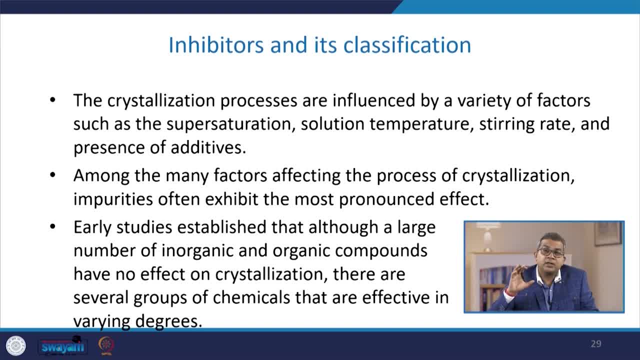 the deposit inhibition. then we have to look into about the concept of inhibitors and how we can classify these inhibitors, because there are different type of scales so we need to have a similar type of classification scheme for inhibitors. So the crystallization processes: 1.. 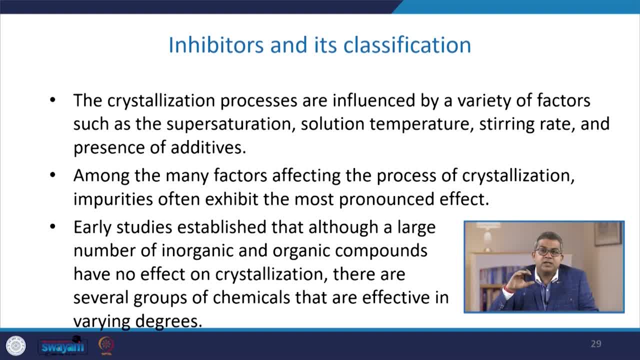 Usually they are influenced by a variety of factors such as supersaturation, solution temperature, sometimes stirring rate, sometimes presence of additives, etc. Among the many factors affecting the process of crystallization, the impurities often exhibits the most pronounced effect. early studies- usually they- established that, although a large 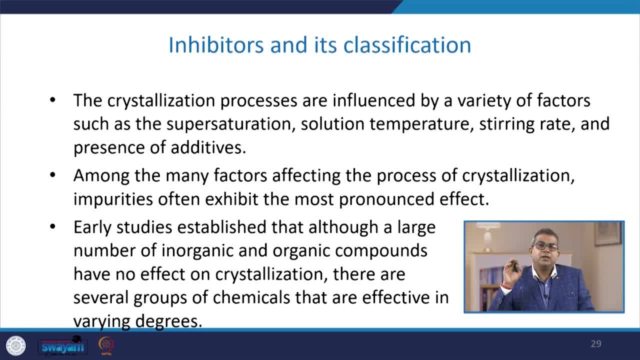 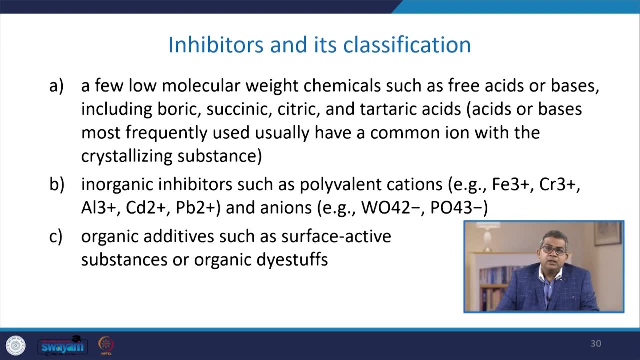 number of inorganic compounds are present in the crystallization process. 2. Inorganic and organic compounds: they have no effect on crystallization. There are several groups of chemicals that are effective in varying degree. when we talk about the classification, very few molecular weight chemicals such as free acids or bases. 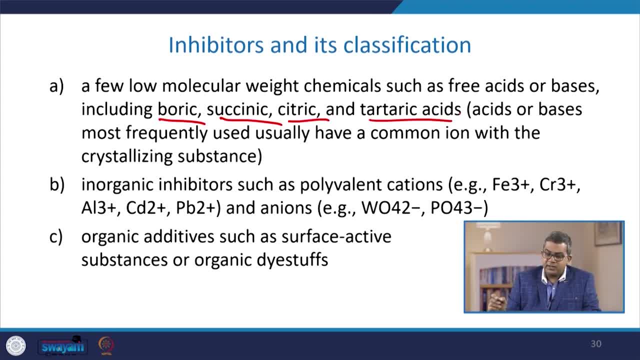 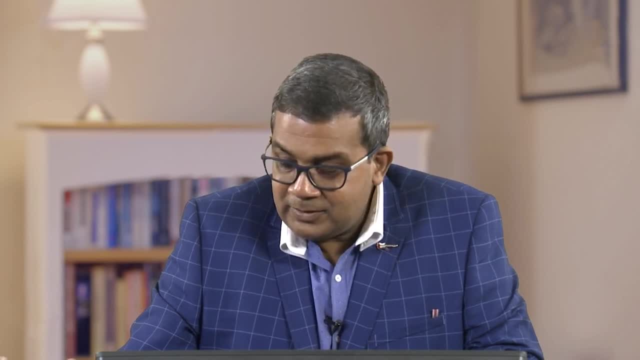 including boric, succinic, citric, tartaric acids, acid or bases most frequently used usually have a common ion with the crystallizing substance. 3. Inorganic inhibitors such as polyvalent cations like Fe3+, Cr3+, Al3+, Cadmium, Lead and anions. 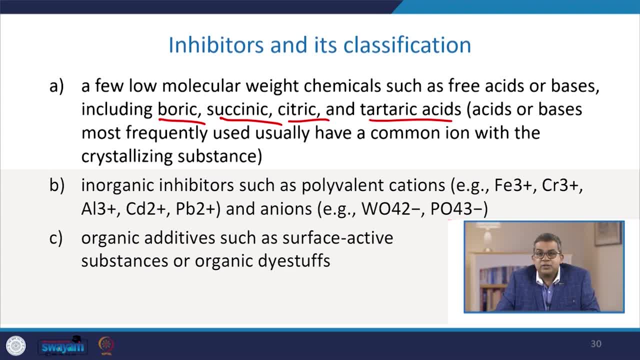 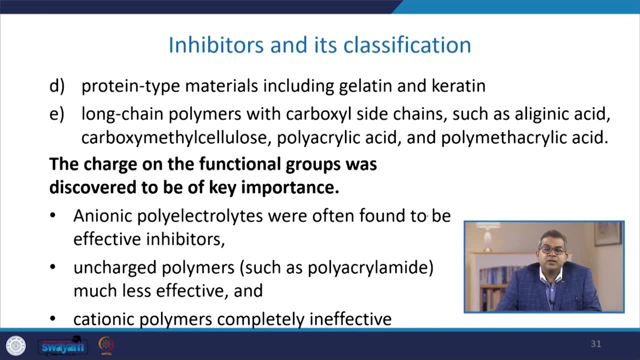 such as tungsten tetroxide and phosphorus tetroxide, etc. 4. Organic additives, such as surface active substance or organic diester. 5. Protein type materials, such as gelatin, keratin, long chain polymers with carboxyl side chains. 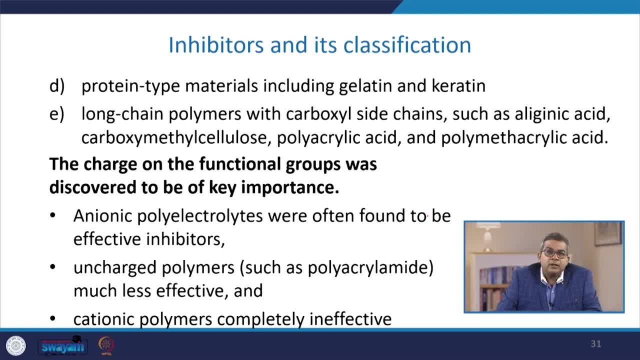 such as allogenic acids, carboxymethyl, cellulose, polyacrylic acid, polymethacrylic acids. 6. The charge on the functional groups usually was discovered to be the key importance. that is very crucial Now. anionic polyelectrolytes were often found to be effective inhibitors. uncharged polymers. 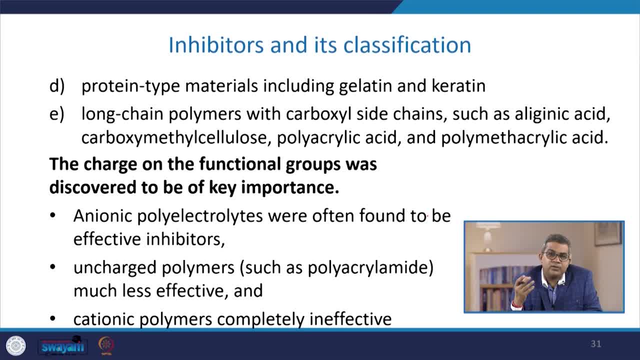 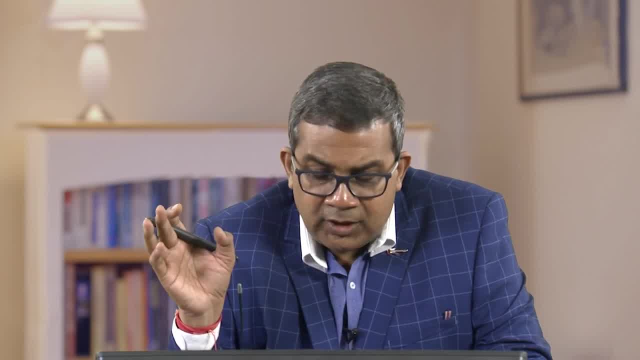 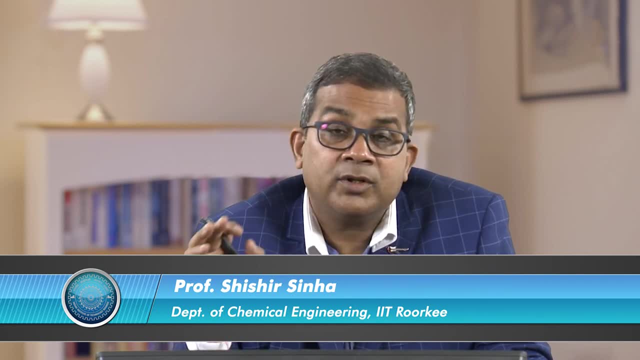 such as polyacrylamide. they are much less effective and cationic polymer completely ineffective. Now let us have a discussion about the mechanism of inhibition, how they work and what is there important, etc. Because this is again very crucial aspect to inhibitors. Now let us have a discussion about the mechanism of inhibition, how they work and what is there important, etc. because this is again very crucial aspect to inhibitors. Now let us have a discussion about the mechanism of inhibition, how they work and what is there. 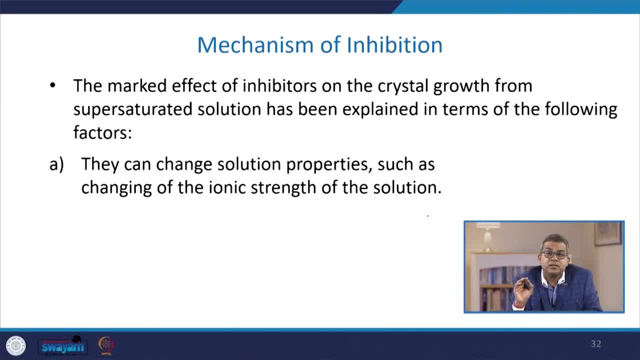 important, etc. because this is again very crucial aspect to inhibitors. Now let us have a discussion about the mechanism of inhibition, how they work and what is there important, etc. because this is again very crucial aspect to inhibitors. Now let us have a discussion about the mechanism of inhibition, how they work and what is there. 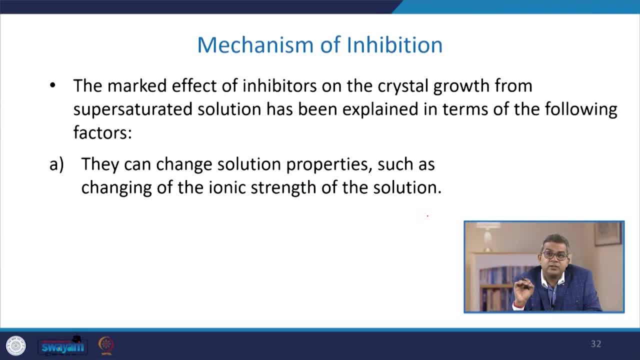 important, etc. because this is again very crucial aspect to inhibitors. Now let us have a discussion about the mechanism of inhibition, how they work and what is there important, etc. because this is again very crucial aspect to inhibitors. Now let us have a discussion about the mechanism of inhibition, how they work and what is there. 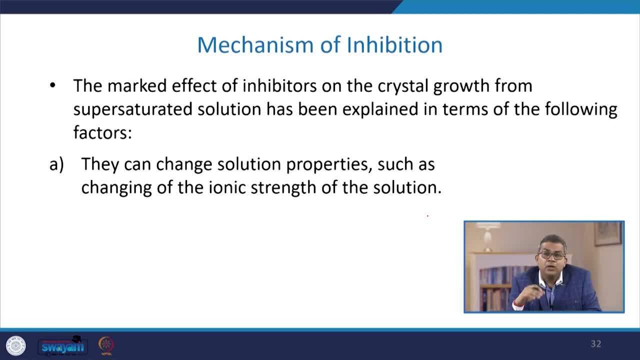 important, etc. because this is again very crucial aspect to inhibitors. Now let us have a discussion about the mechanism of inhibition, how they work and what is there important, etc. because this is again very crucial aspect to inhibitors. Now let us have a discussion about the mechanism of inhibition, how they work and what is there. 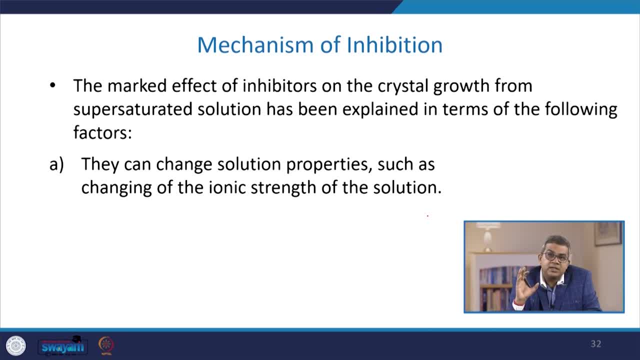 important, etc. because this is again very crucial aspect to inhibitors. Now let us have a discussion about the mechanism of inhibition, how they work and what is there important, etc. because this is again very crucial aspect to inhibitors. Now let us have a discussion about the mechanism of inhibition, how they work and what is there. 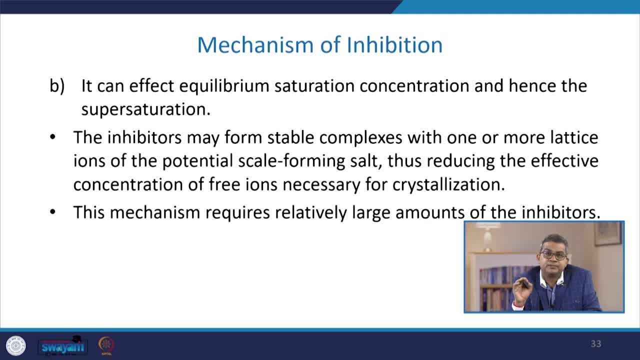 important, etc. because this is again very crucial aspect to inhibitors. Now let us have a discussion about the mechanism of inhibition, how they work and what is there important, etc. because this is again very crucial aspect to inhibitors. Now let us have a discussion about the mechanism of inhibition, how they work and what is there. 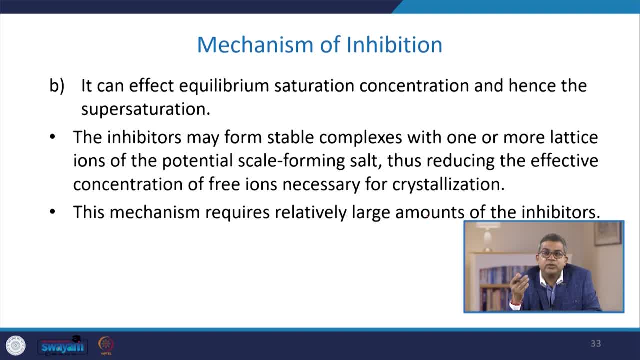 important, etc. because this is again very crucial aspect to inhibitors. Now let us have a discussion about the mechanism of inhibition, how they work and what is there important, etc. because this is again very crucial aspect to inhibitors. Now let us have a discussion about the mechanism of inhibition, how they work and what is there. 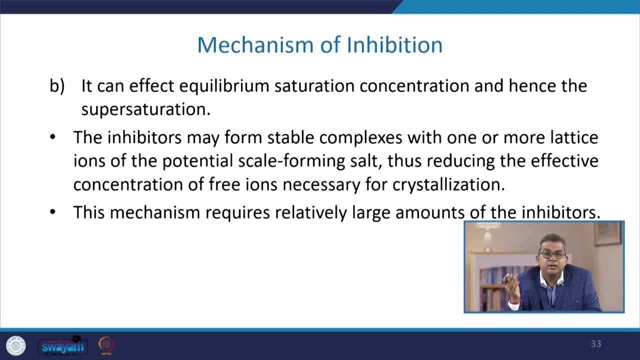 important, etc. because this is again very crucial aspect to inhibitors. Now let us have a discussion about the mechanism of inhibition, how they work and what is there important, etc. because this is again very crucial aspect to inhibitors. Now let us have a discussion about the mechanism of inhibition, how they work and what is there. 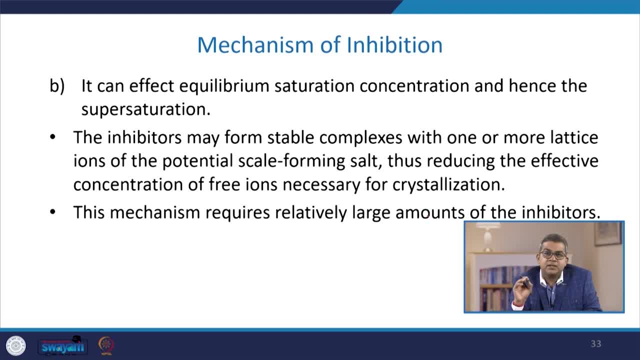 important, etc. because this is again very crucial aspect to inhibitors. Inhibitors may form stable complexes with one or more lattice ions of the potential scale forming salt, therefore reducing the effective concentration of free ion necessary for crystallization. This mechanism requires relatively large amount of inhibitors. 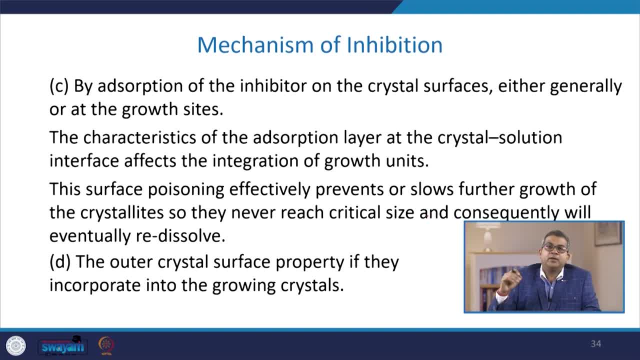 Another is by adsorption of the inhibitor on the crystal surface. they are either generally on or at the growth sites. The characteristics of absorption layer at the crystal solution interface affects the integration of growth unit- This surface poisoning, usually termed as a surface poisoning. this effectively prevents 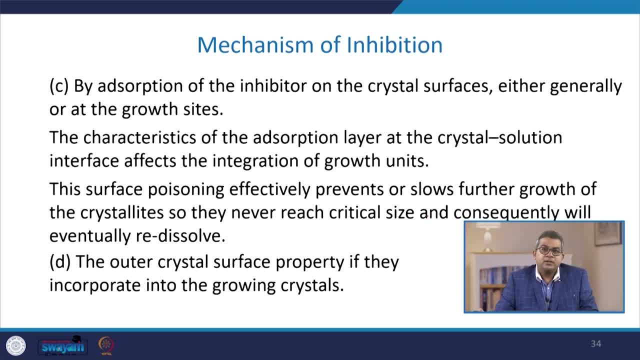 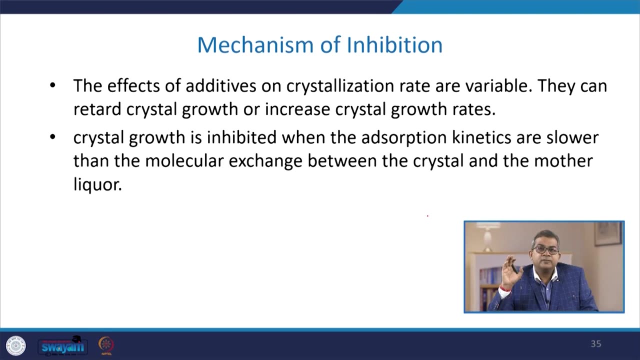 or slows further growth of the crystallites so they never reach the critical size and consequently will eventually be damaged. So it creates a barrier between the surface and the targeted sites, The outer crystal surface property, if they incorporate into the growing crystal the 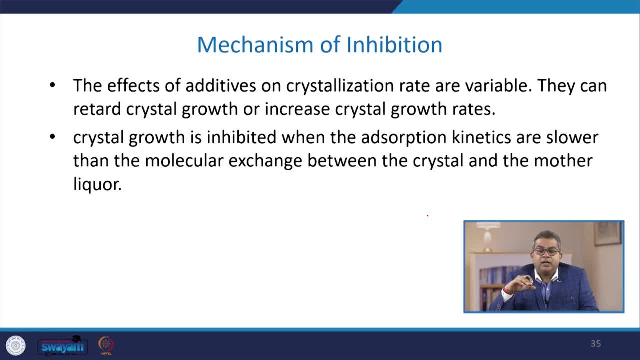 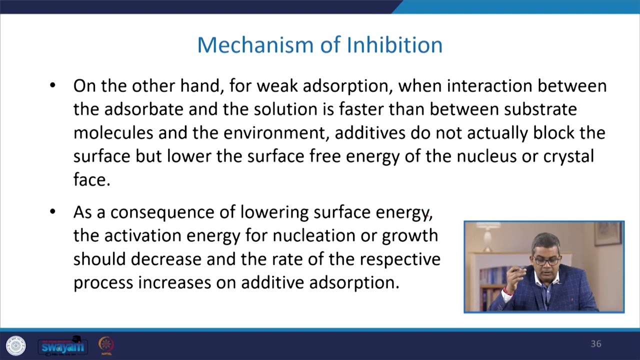 effect of additives on crystallization rate are variable. They can retard the crystal growth or sometimes increase the crystal growth rates. Crystal growth is a very important factor. Crystal growth is usually inhibited when the adsorption kinetics are slower than the molecular exchange between the crystal and the mother liquor. 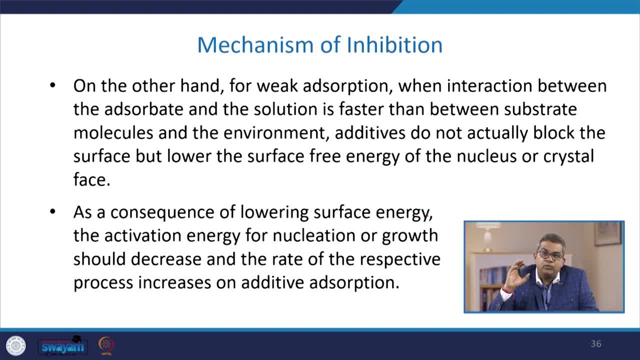 On the other hand, for weak adsorption, when interaction between the adsorbate and the solution is faster than between the substrate molecules and the environment, additives do not actually block the absorption. They block the surface, but they lower the surface free energy of the nucleus or crystal. 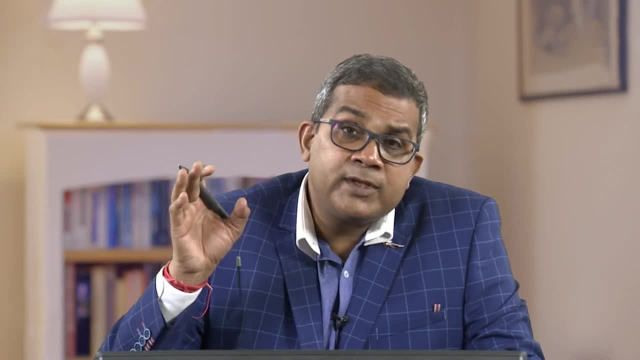 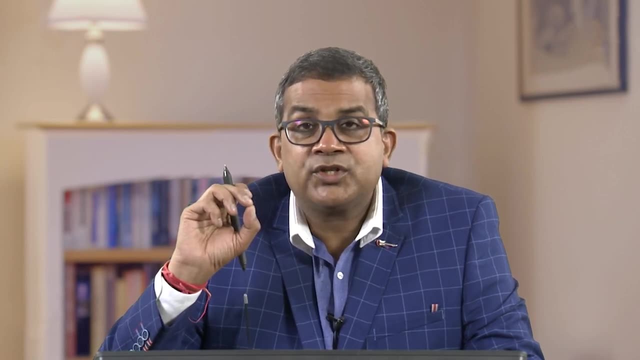 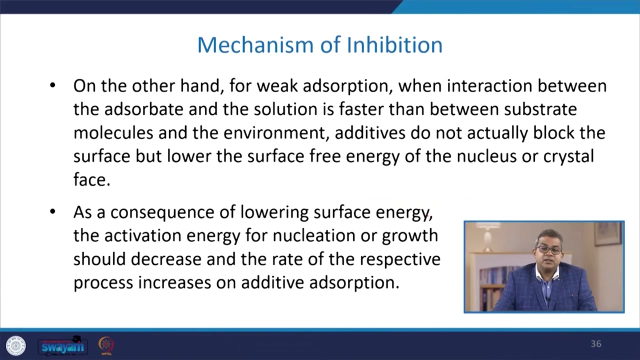 phase. So the knowledge about the surface free energy is important because this is again the key factor of scale inhibition in this particular category. So as a consequence of lowering surface energy, the activation energy for nucleation or growth, it should decrease and the rate of respective process increases. on additive adsorption: 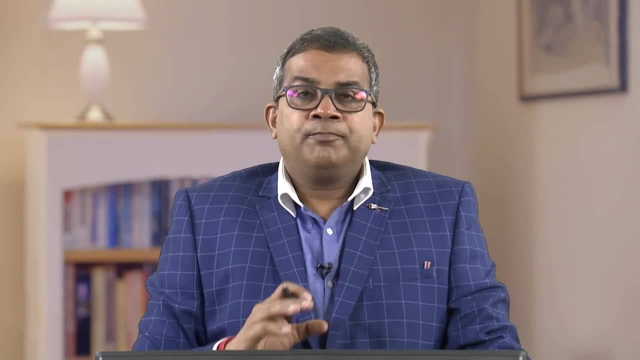 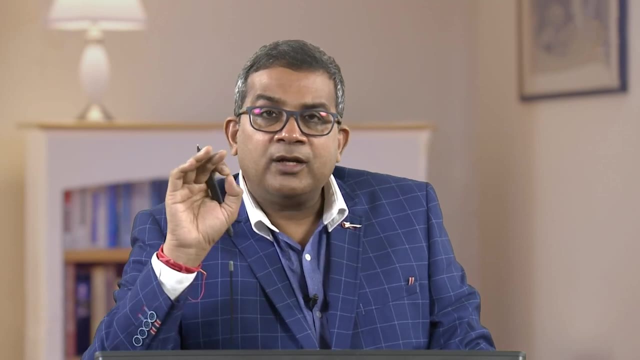 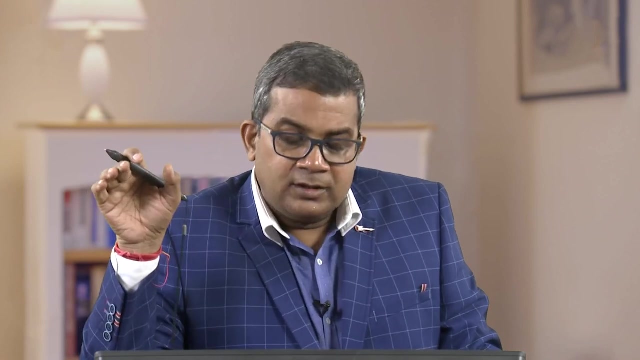 So earlier it was reported that the additive both promotes growth at a low concentration and retard growth at high concentration in the same system. In most cases, the presence of additive reduces the overall crystallization rate, So this is a very important factor. 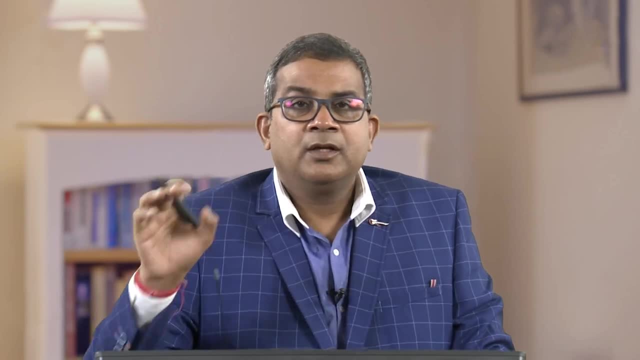 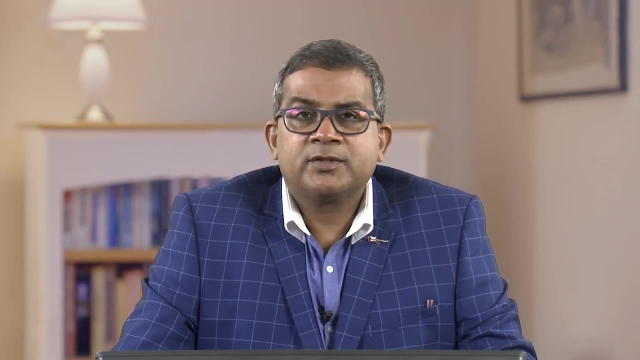 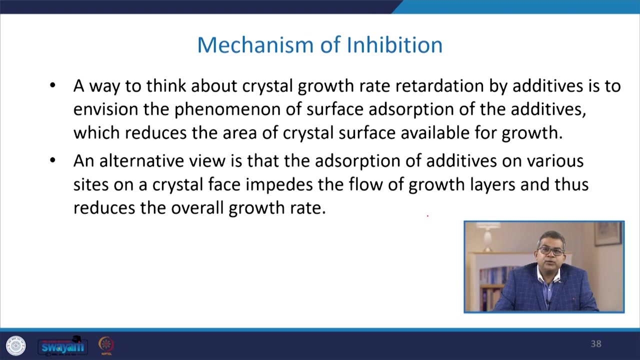 Overall crystal growth rate. A way to think about the crystal growth rate retardation, usually by the additives, is to envision the phenomena of surface adsorption of the additives, which in situ reduces the area of crystal surface available for growth. An alternative view is that the adsorption of additives on various sites, such as the. 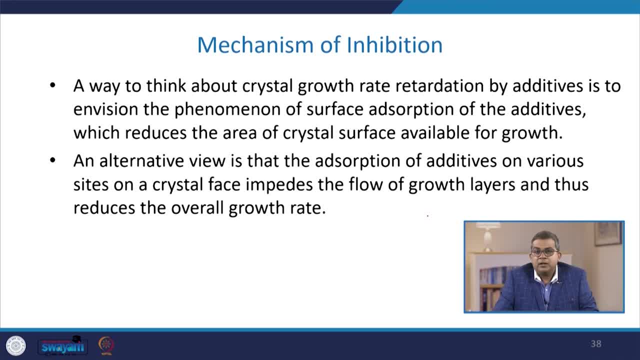 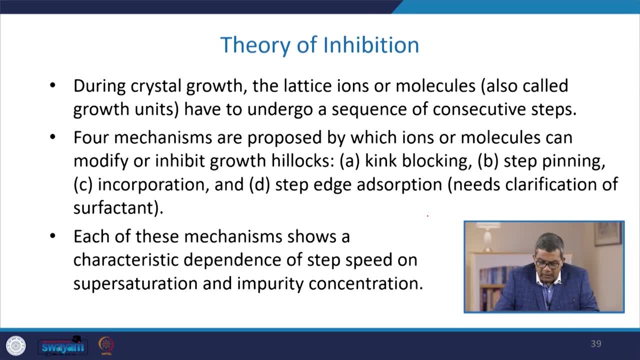 deposits on crystal phase impedes the flow of growth layer and therefore reduces the overall growth rate. Now let us discuss about the theory of inhibition. Now, during crystal growth, the lattice ion or molecules- they are also called the growth units- they have to undergo a sequence of consecutive steps. 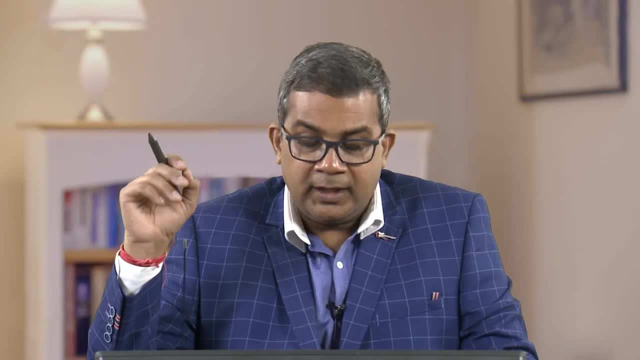 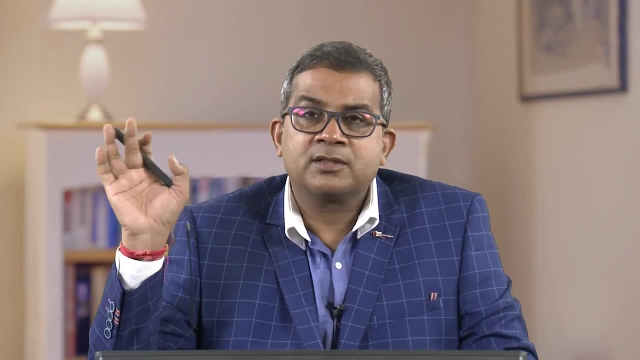 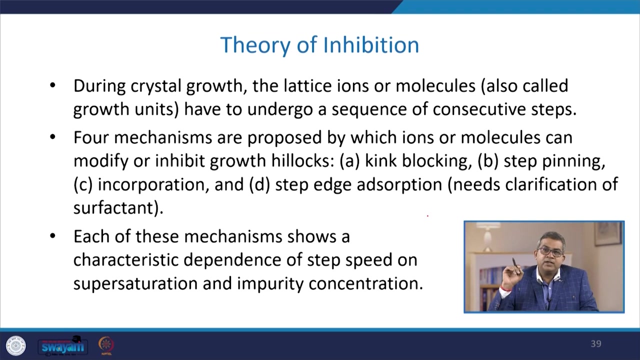 So people have suggested the four mechanisms: The first mechanism by which ions or molecules they can modify or inhibit growth, helox. One is kink blocking. other is the step pinning. the third one is incorporation. and fourth one is the step age adsorption. 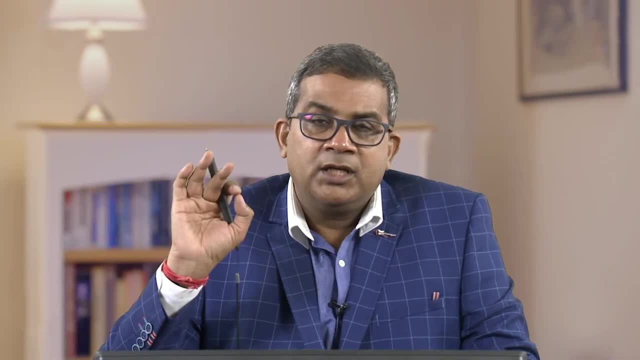 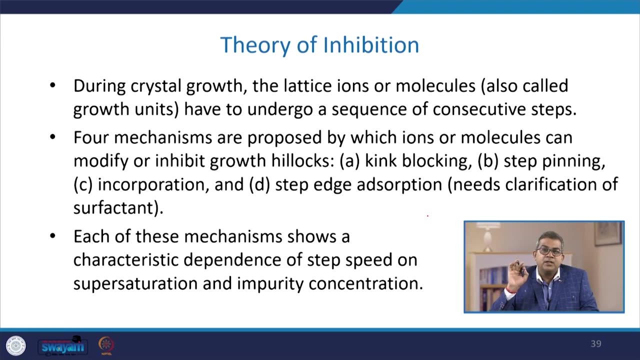 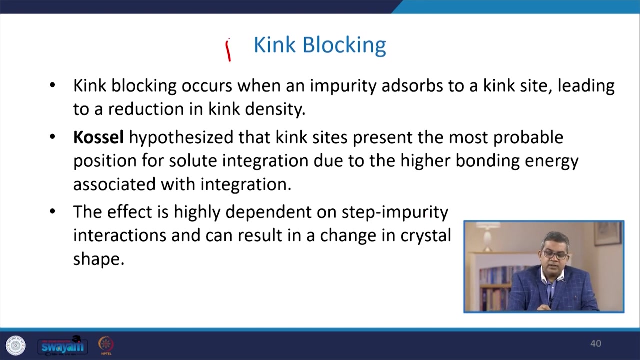 This needs the clarification of surfactant. Each of these mechanisms shows a characteristics dependence of step speed on the adsorption of surfactant. So let us take the first one, that is, the kink blocking. Now, kink blocking occurs when an impurity adsorbs to the kink site, leading to a reduction. 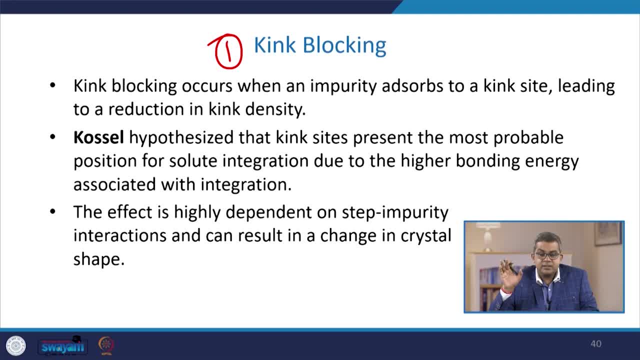 in kink density. Kossel hypothesized that the kink sites present the most probable position of for solute integration, due to higher bonding energy associated with kink. So this is the first one. Let us take the second one. 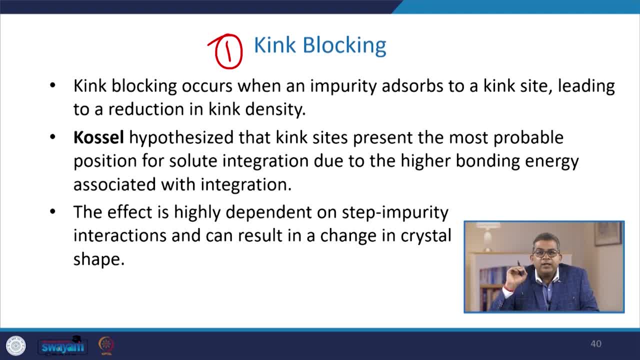 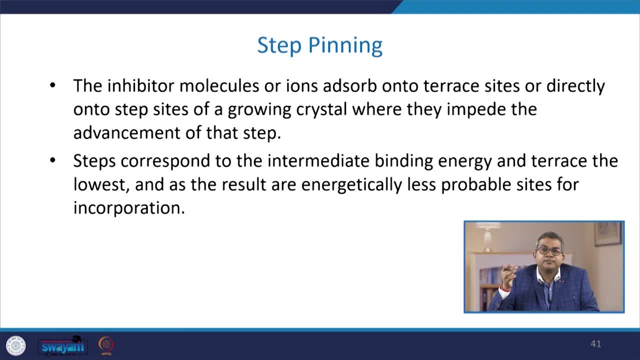 This is the step integration, The effect of highly dependent on step impurity interaction and can result in change in crystal shape. Next is step pinning. that is number 2.. The inhibitor molecules or ions adsorbed onto the terrace site or directly onto step sites. 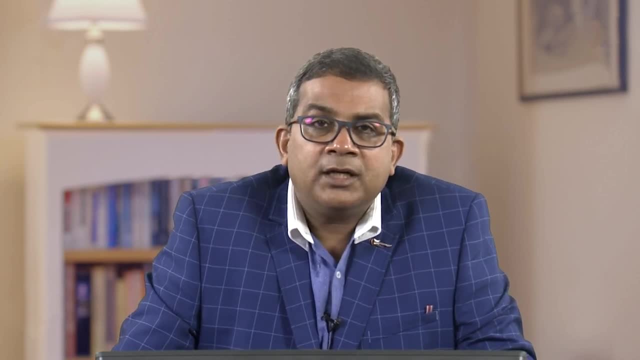 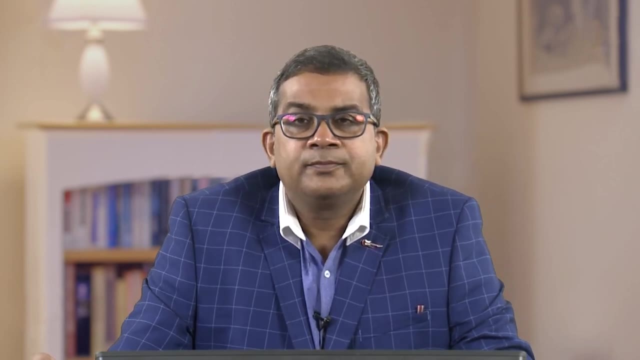 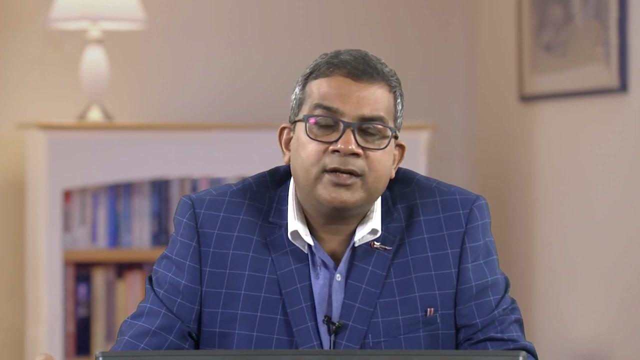 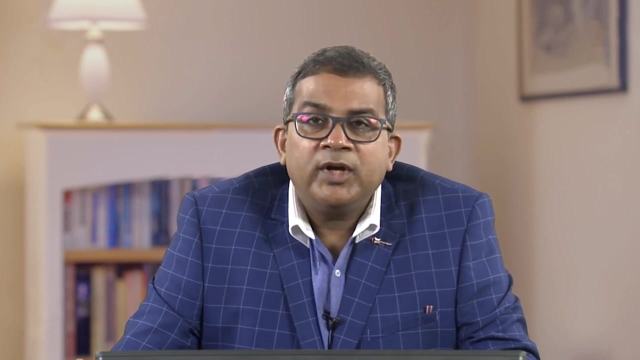 of growing crystal, where they impede the advancement of that step. Now, step correspond to the intermediate binding energy and terrace, the lowest and as the result are energetically less probable site available for incorporation. The step is, however, is able to move around and squeeze through the neighboring inhibitors. 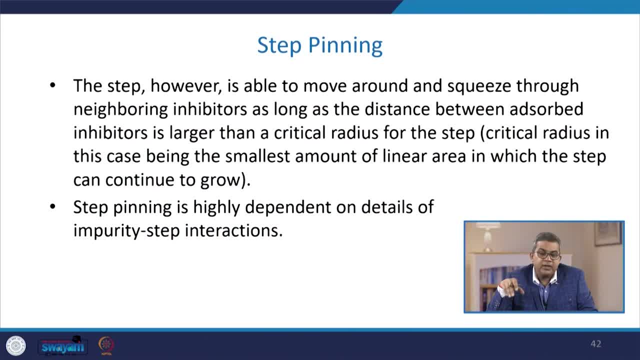 as long as the distance between adsorbed inhibitors is larger than a quarter. So this is the step integration. Now let us take the third one. This is the step integration: The effect of highly dependent on step impurity interaction and can result in change in crystal.